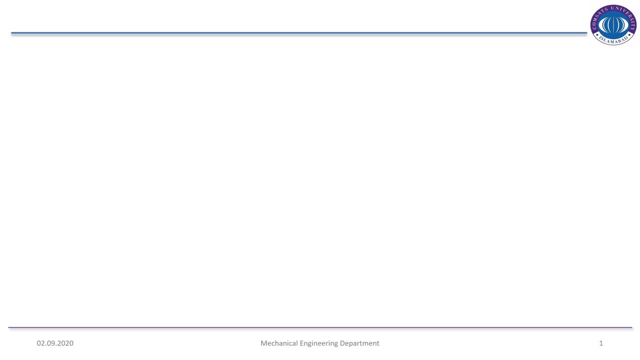 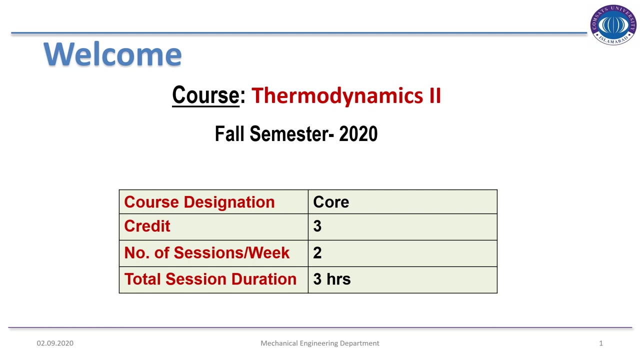 Assalamu alaikum, dear students, I hope you are all fine by the grace of Almighty Allah. I welcome you all to the course of Thermodynamics II, Fall Semester 2020.. Core Designation: It's a core course. It's a three credit hour course. Number of sessions per week will be two. Total session duration will be three hours. 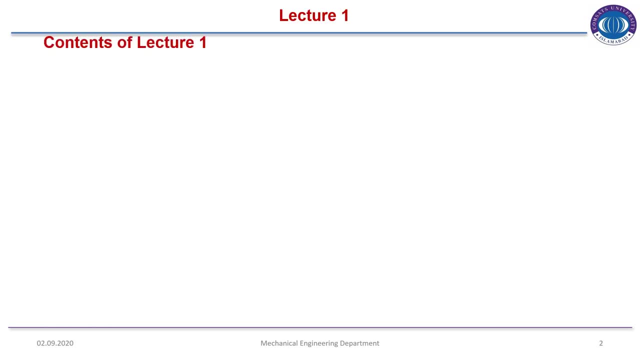 This is our lecture one. Contents of lecture one are discussion of lesson plan and discussion of important topics of Thermodynamics I. These topics include thermodynamics and energy system and control volume properties of system, state and equilibrium processes and cycles, temperature scales and pressure. 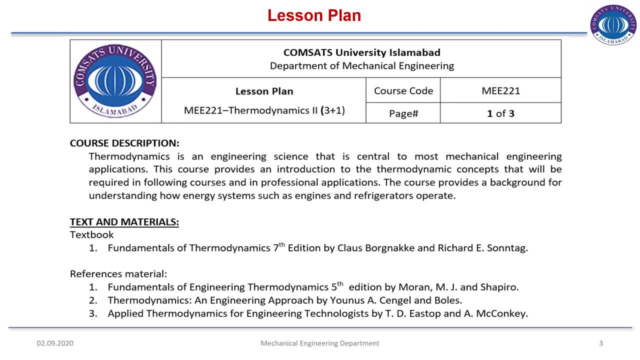 Lesson Plan. This is the lesson plan of Thermodynamics II. Course Description. Thermodynamics is an engineering science that is central to most mechanical engineering applications. This course provides an introduction to the thermodynamic concepts that will be required in following courses and in professional applications. 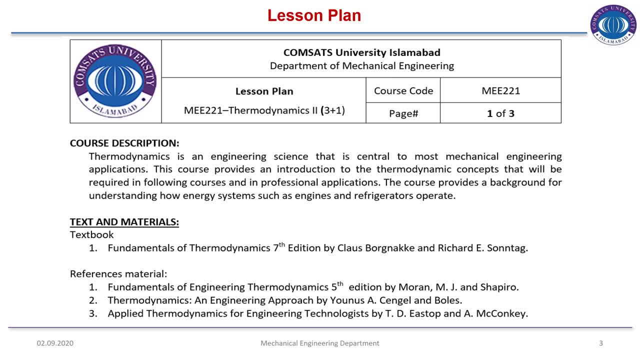 The course provides a background for understanding how energy systems such as engines and refrigerators operate, So like in the subject of IC engine heat transfer, refrigeration and air conditioning power plant, All these courses that you will be studying in future semester are the application of thermodynamics. 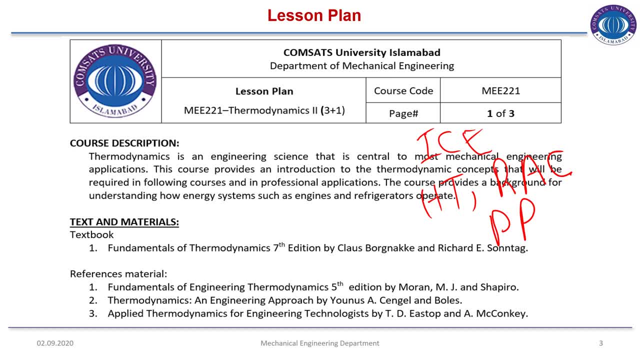 Test Book. The test book which we will be following is the Fundamentals of Thermodynamics by Brognac and Sontag, 7th edition. Reference material will be Fundamentals of Engineering. Fundamentals of Engineering Thermodynamics, 5th edition by Shapiro. 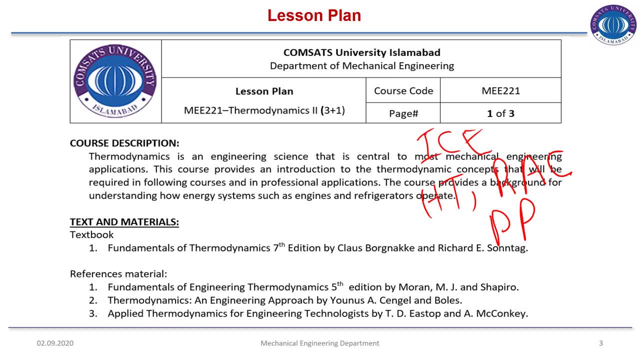 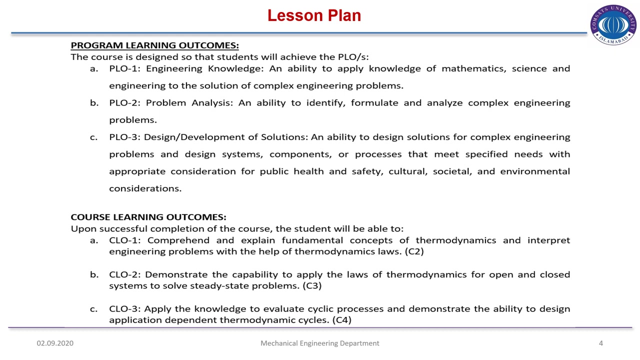 Thermodynamics and Engineering Approach by Sanger. Applied Thermodynamics for Engineering Technologists by McConaughey. The first book is our test book and all other books are the helping material which we will be using for our discussion, And some of the numerical that are in the lecture are from the reference material as well. 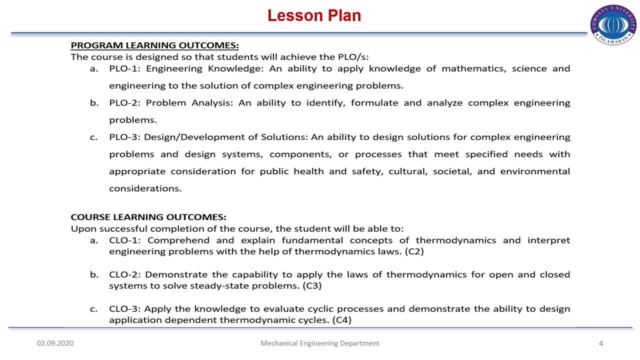 Lesson Plan: Program Learning Outcome. There are three program learning outcomes: PLO1, PLO2 and PLO3.. PLO1 is Engineering Knowledge: An ability to apply knowledge of mathematics, science and engineering theory To the solution of complex engineering problems. 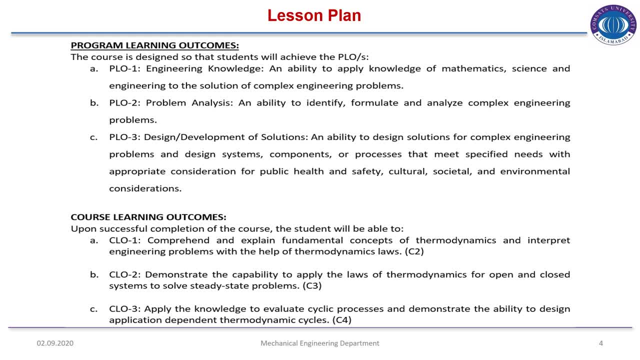 PLO2, Problem Analysis: An ability to identify, formulate and analyze complex engineering problems. PLO3, Design and Development of Solutions: An ability to design solutions for complex engineering problems and design systems, components or processes that meet specified needs, With appropriate consideration for public health, safety, cultural, societal and environmental concerns. 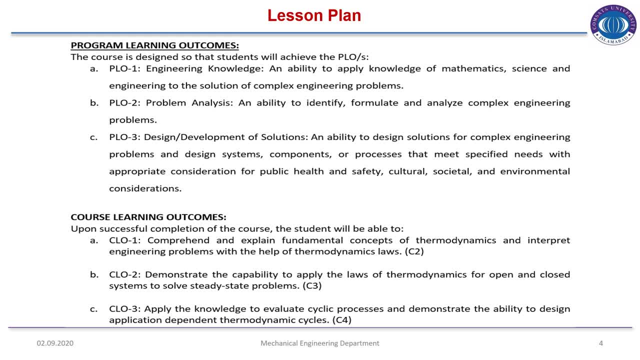 Course Learning Outcomes. There are three course learning outcomes: CLO1,, CLO2, CLO3.. CLO1, Comprehends and explains fundamental concepts of thermodynamics and interprets engineering problems with the help of thermodynamic laws. 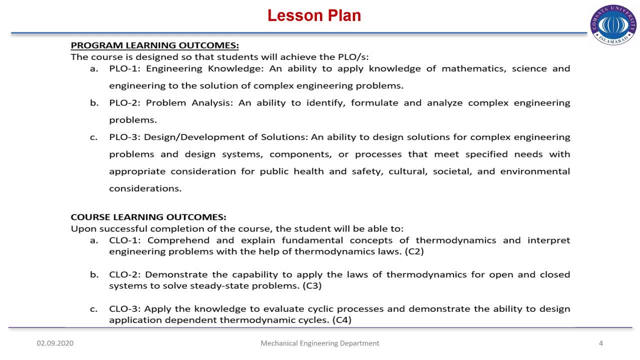 Course Learning Outcome: 2. Demonstrates the capability to apply the laws of thermodynamics for open and closed systems to solve steady state problems. CLO3, Applies the knowledge to evaluate the science and engineering problems. CLO4, Applies the knowledge to evaluate the cyclic processes and demonstrate the ability to design application-dependent thermodynamic cycle. 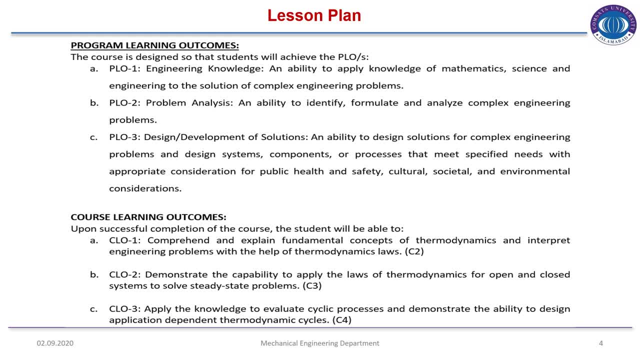 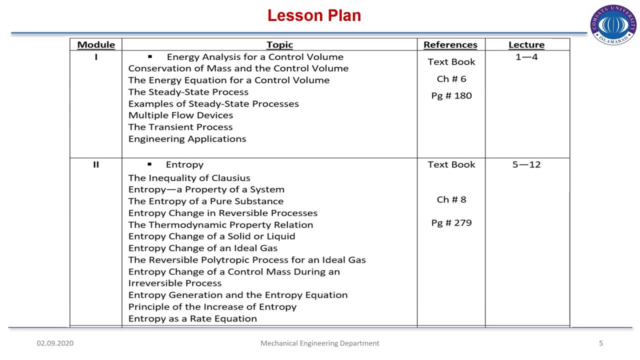 Course Learning Outcomes. There will be total of five modules that we will be studying in the course of Thermodynamics 2.. In module 1, there will be energy analysis for control volume. Course Learning Outcomes: Conservation of mass and control volume. 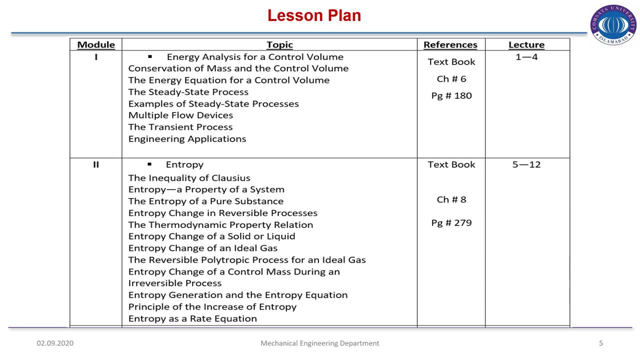 The energy equation for control volume. The steady state processes- Example of steady state processes: Multiple flow devices. The transient processes, Engineering applications In the textbook of Broknack. this is chapter 6, page number 180.. Course Learning Outcomes. 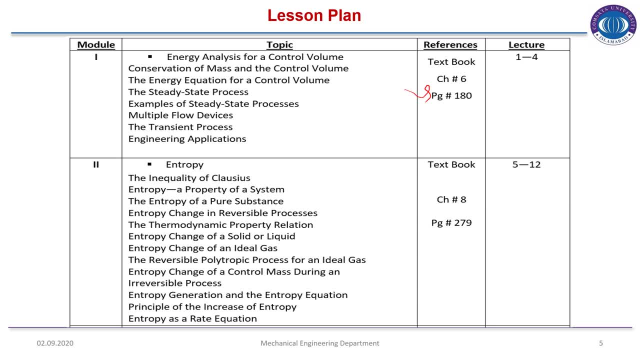 In module 2, the name of the chapter is Entropy- The equality of Clausius. Entropy a property of system. The entropy of pure substance. Entropy change in reversible processes. The thermodynamic property relation. Entropy change of solid and liquid. 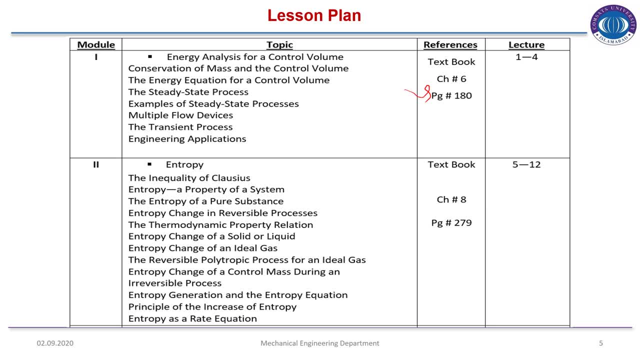 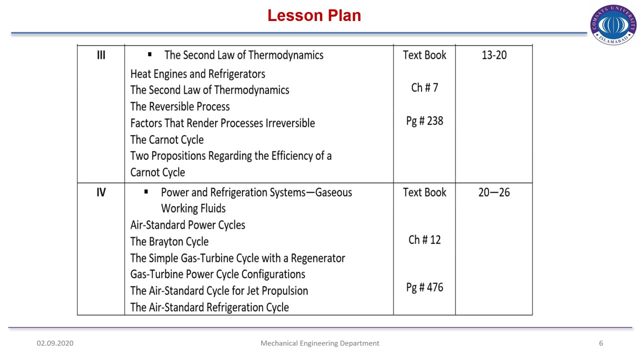 Entropy change of an ideal gas. The reversible polytropic process for an ideal gas. Entropy change of a controlled mass during an irreversible process. Entropy generation and entropy equation. Principle of increase of entropy Entropy as a rate of equation. 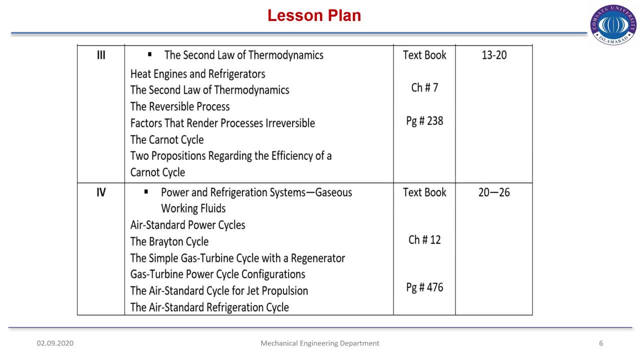 Module 3.. The second law of thermodynamics: Heat engines and refrigerator. The second law of thermodynamics: The reversible processes- Factors that render process irreversible. The Carnot cycle. Two propositions regarding the efficiency of Carnot cycle. This is chapter 8, page 238 of our textbook. 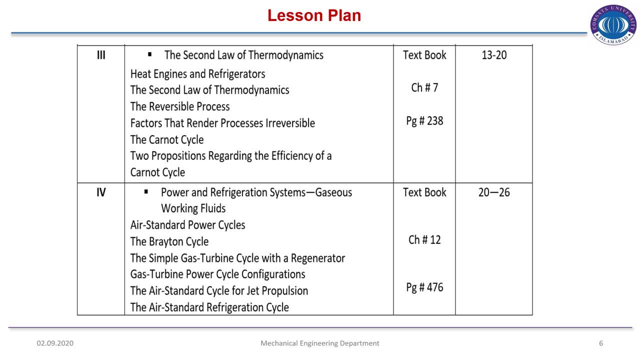 Power and refrigeration system. Gaseous working fluid- Module 4.. The content of module 4 are: air standard power cycles, The Brayton cycle, The simple gas turbine cycle with regenerator Gas turbine power cycle configurations. The air standard cycle for jet propulsion. 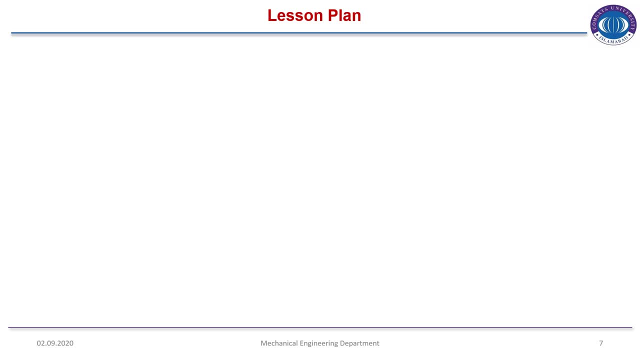 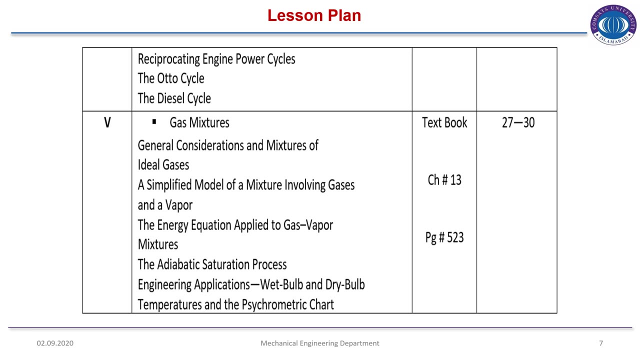 The air standard refrigeration cycle, Reciprocating engine power cycles, The auto cycle And the diesel cycle. This is chapter 12 of our book. The module 5 is general consideration of mixture Ideal gases, A simple model of mixture involving gases and vapor. 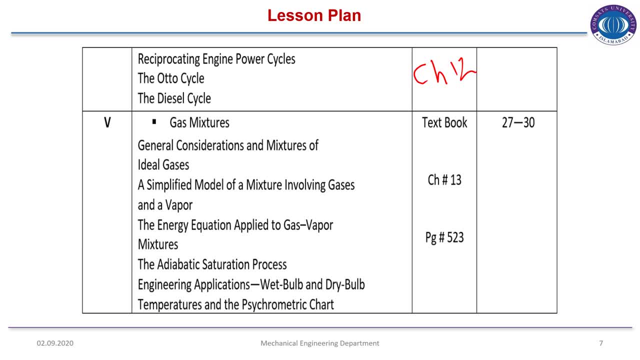 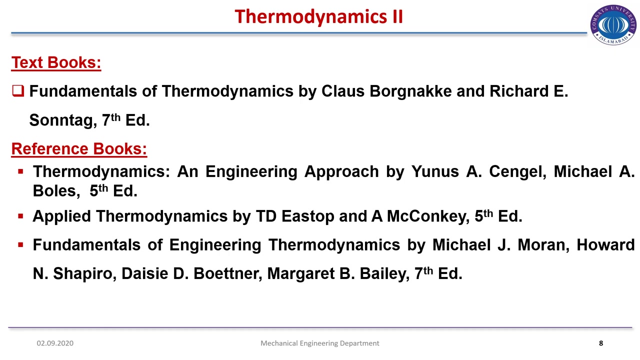 The energy equation applied to gas vapor mixture, The adiabatic saturation process, Engineering applications, Wet bulb and dry bulb, Temperatures and psychometric charts. This is chapter 13 of our textbook, page 523.. As already discussed, this is our textbook, which we will be following. 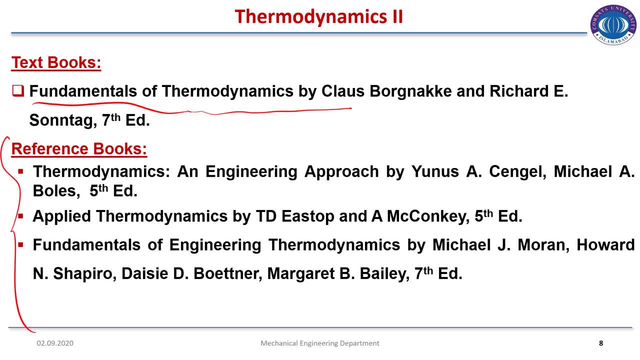 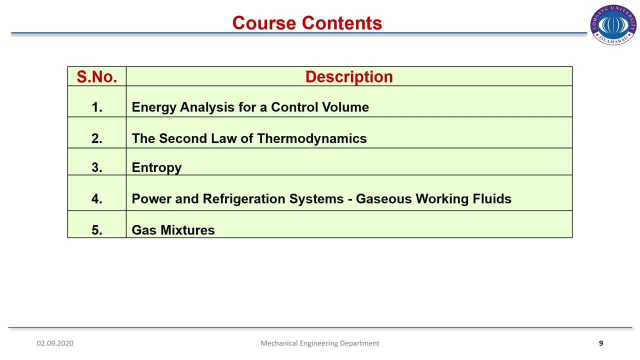 And these are our reference material. This is our course content: Energy analysis of control volume. By control volume we will mean that open system, Energy analysis of a open system, The second law of thermodynamics, Entropy Power and refrigeration system. 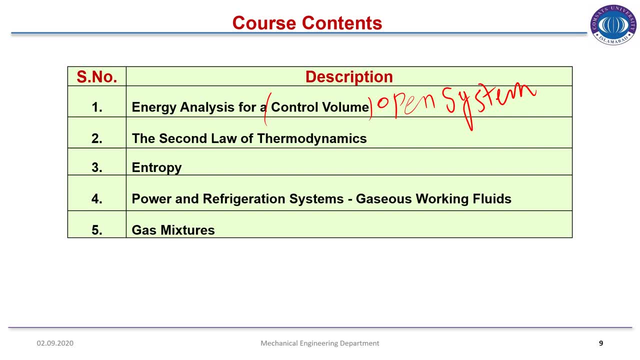 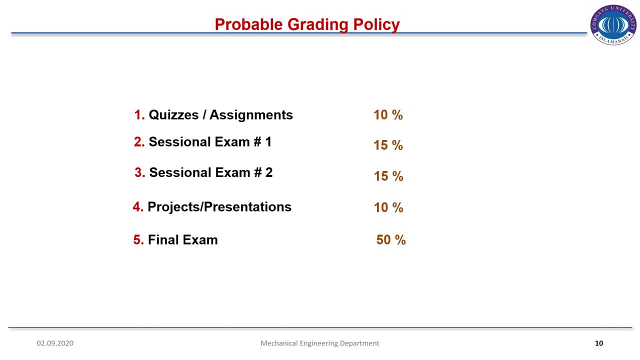 Gaseous working fluid And gas mixture, The całe of the thermal body And the energy field. Theruck And caustic acid And carbon dioxide, The구ick, And the solution to the problem, The second law of thermodynamics. 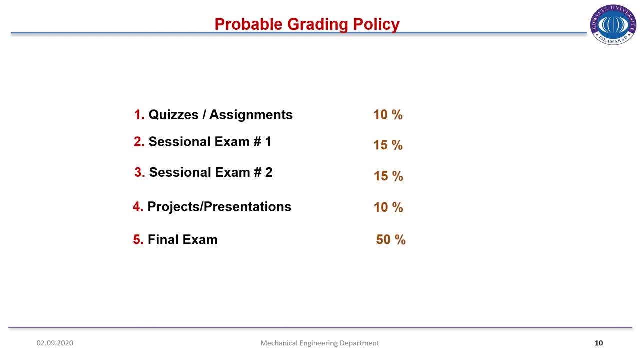 The equation for switching weapons. The equation is given by a transformation equation And you can see the calculation of the butane And you have to make the subtracted function And you have to write the expression And you have to make the subtracted function. 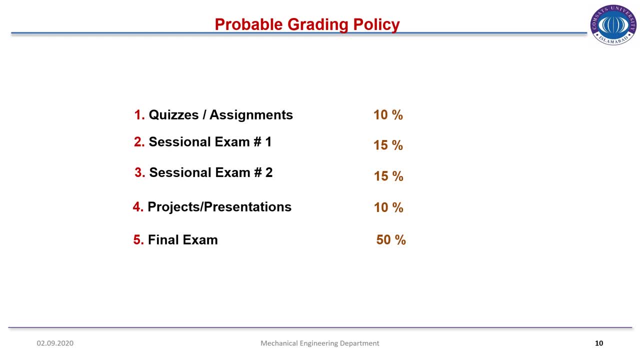 And you can use the function And you have to use the function. We are going to do that in a minute. However, we can also do that later in this class, But that was my only consideration, So we are going to discuss that later. 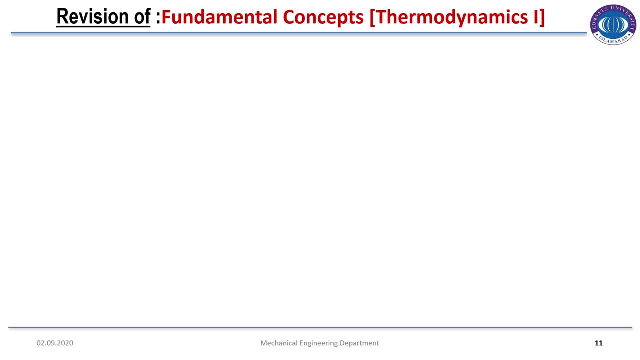 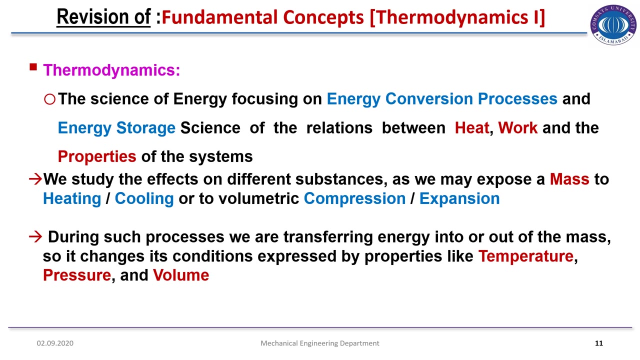 If you have any further questions, You can call us on our website And let us know in the comments. revision of fundamental concepts of thermodynamics. one okay. thermodynamics focus on the energy conversion process, energy storage and its drive relation between heat work and properties of the 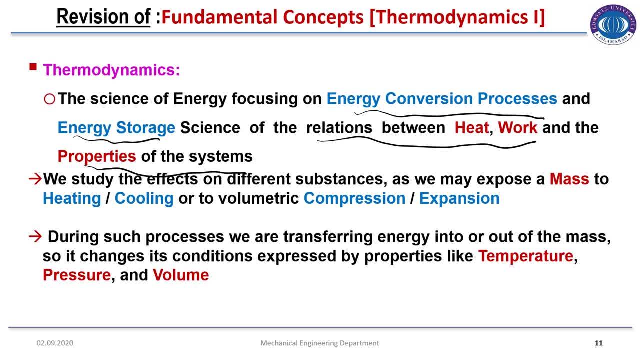 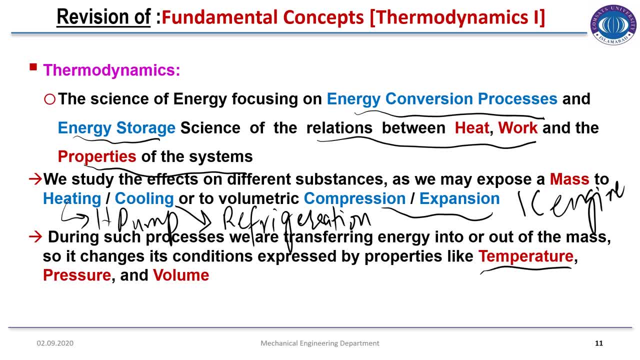 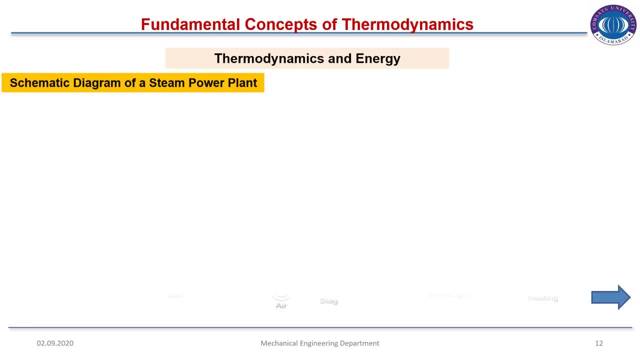 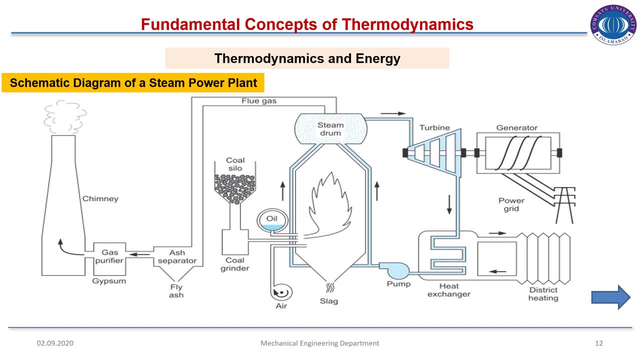 properties like temperature, pressure and volume. this is the schematic diagram of steam. this is the schematic diagram of steam power plant power plant coal will be inserted in the power plant through coal silo. contains chemical energy. through the process of combustion the chemical energy will be converted into. 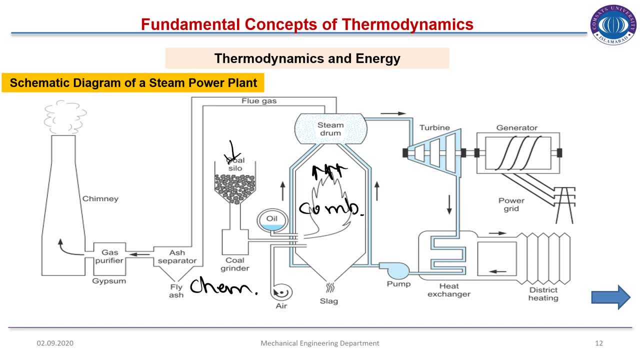 heat energy which will transfer heat to water stored in the drum and convert it into hot, high-pressure, high energy steam which will strike at the turbine blades which is connected to the generator, which is connected to the generator. the generator will produce electricity. low pressure, low energy stream will come into heat exchanger. 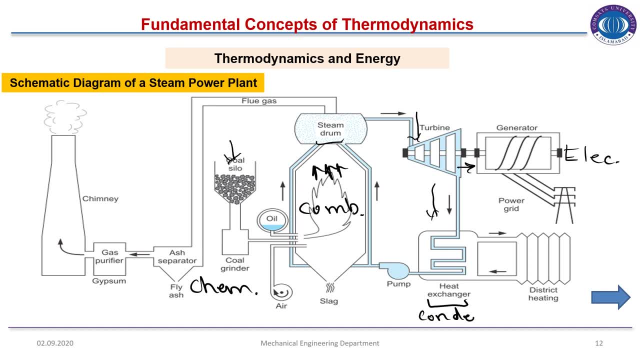 and in the process of condensation you can see caramel sesame seedا. bottle of gas actiam vat. The energy will be emitted, taken out from the steam and it will be used as the stick heating. The steam will be converted into liquid and the pump will push the liquid back into the drum. 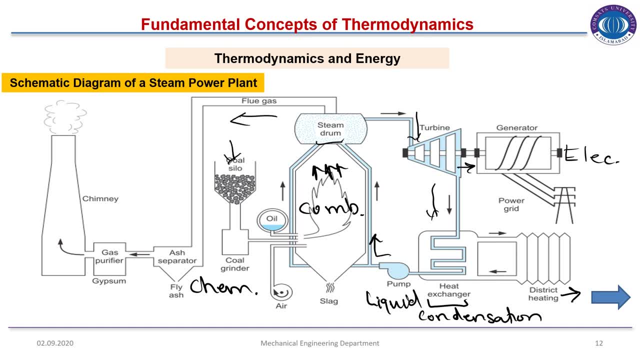 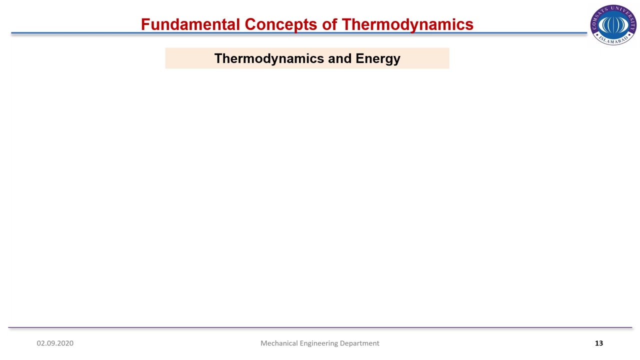 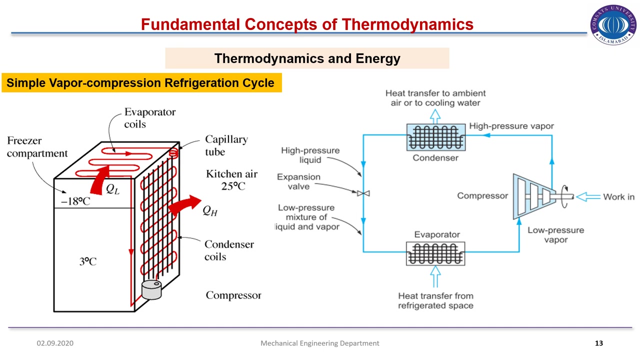 These are the flue gases which will be produced due to the process of combustion and, upon purification, these gases will be emitted into the theory. Simple vapor compression refrigeration cycle. this is a fridge- household fridge. This is the cabinet of the fridge. At the top of the cabinet you can see multiple tubes that are the vapor coils. 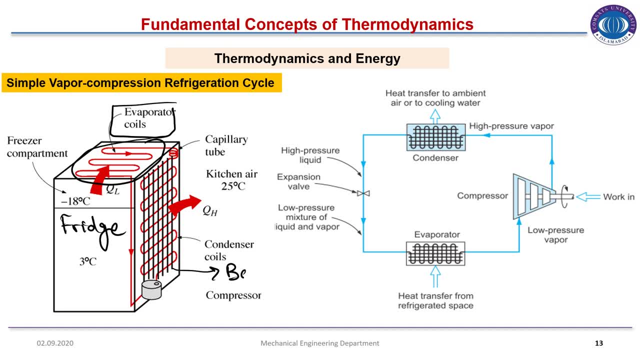 This is the back of the fridge. At the bottom you can see the compressor. The multiple coils that you see at the back of the fridge are the condenser coils. This is the flow cycle shown For vapor compression refrigeration cycle. Low pressure refrigerant is introduced into the compressor, which converts into high pressure vapor. 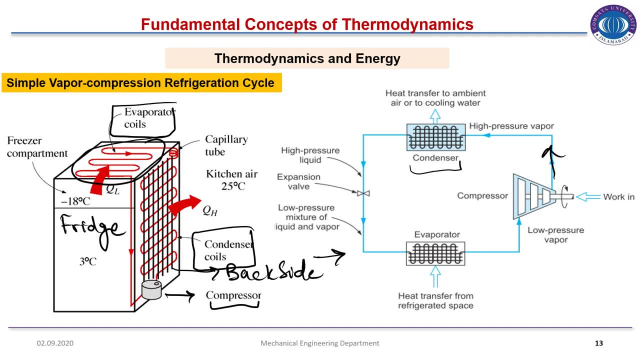 There is a condenser coil, which is shown here at the back side of the fridge. Heat transfer to the ambient air, to the cooling refrigerant. So here the high temperature refrigerant is entering into the condenser and low temperature refrigerant is exiting out. 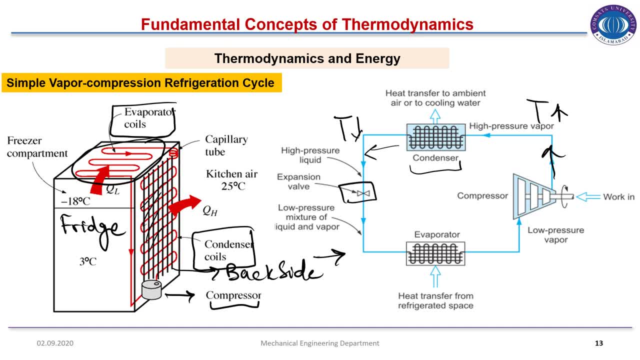 There is an expansion valve which will also lower the pressure of the refrigerant. So low temperature And low pressure refrigerant enters into the evaporator And the heat from the inside space of the fridge will be exchanged through the evaporator And the inside temperature of the fridge will be lowered. 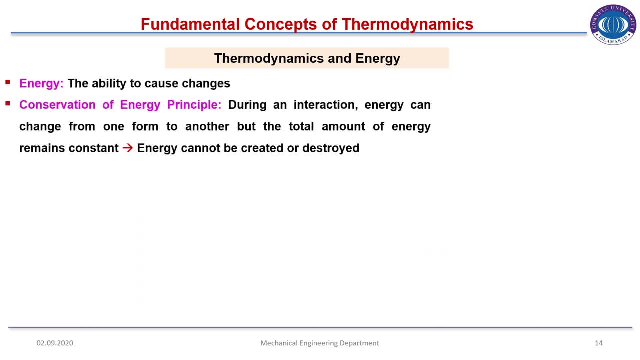 Thermodynamics and energy. There are some basic definitions: Energy: the ability to cause change. Conservation of energy. principle: During an interaction, energy can change from one form to another, But the total amount of energy remains constant. Energy cannot be created or destroyed. 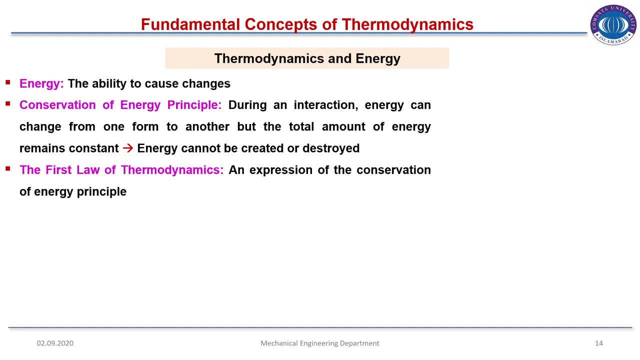 The first law of thermodynamics, An expression of the conservation of energy principle, That is, energy can neither be created nor be destroyed, But it can change from one form to another form. So mechanical energy can be converted into thermal energy and vice versa. 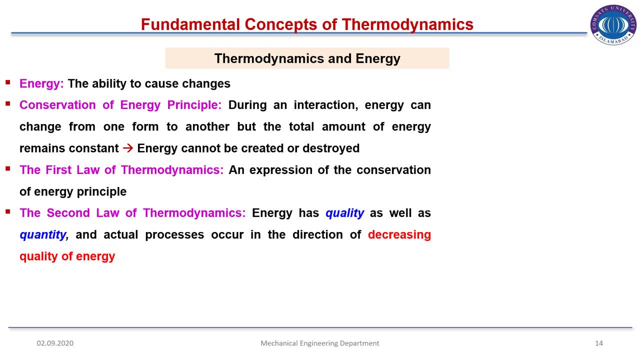 The second law of thermodynamics. Energy has qualitative as well as quantitative, and actual process occur in the direction of decrease of quality of energy. That is why the first law is also known as the quantitative law And the second law is also known as the qualitative law. 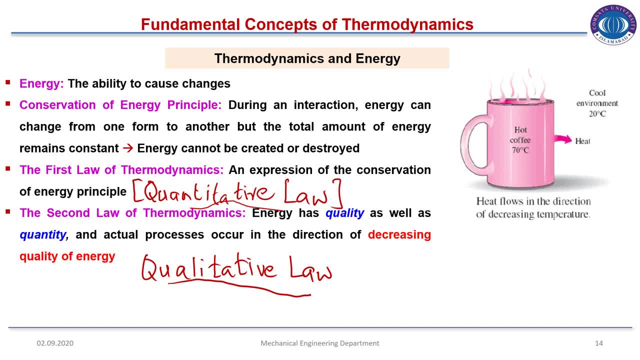 On the right side you can see a hot cup of coffee that is at 70 degrees centigrade. Temperature of the environment is 20 degrees centigrade, So there will be a heat transfer from coffee to the environment through the wall of the cup. 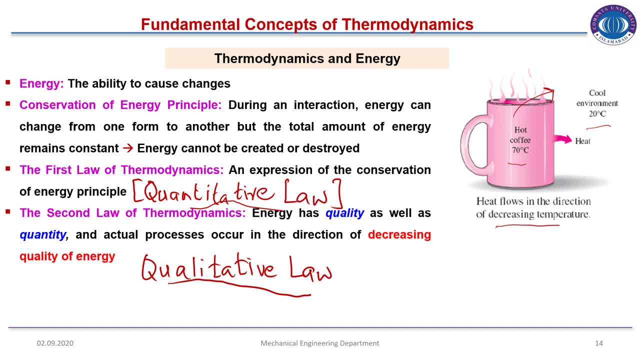 Heat flow in the direction of increase in temperature. Greater energy flow, Greater energy input, will produce a greater energy output. For example, greater energy input food than the energy output. exercise will gain weight, Stored energy in the form of fat, And the person who has smaller energy input than the output will lose weight. 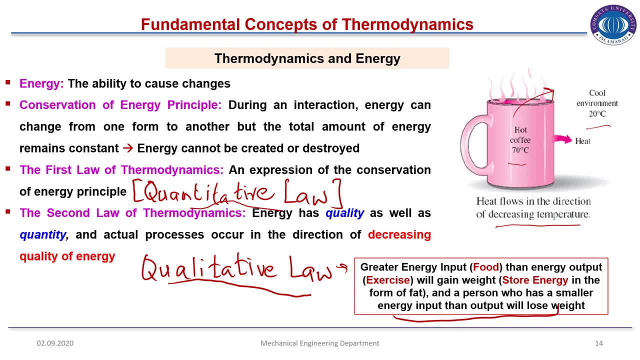 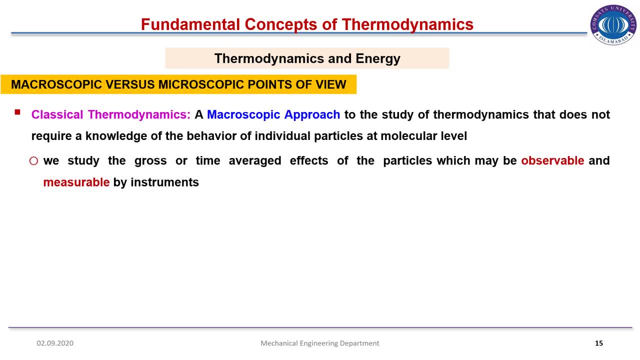 The second law of thermodynamics: Energy can be converted into thermal energy. That is why the first law of thermodynamics: Energy can be converted into thermal energy. through the wall of the cup, Heat flow in the direction of decrease in temperature. The second law of thermodynamics: 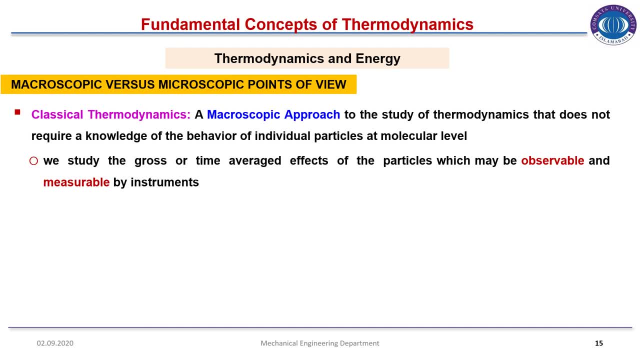 Microscopic versus microscopic points of view. There are two main branches of thermodynamics. One is classical thermodynamics And the other is statistical thermodynamics. Classical thermodynamics deals with the macroscopic approach, Whereas statistical thermodynamics deal with the microscopic approach. 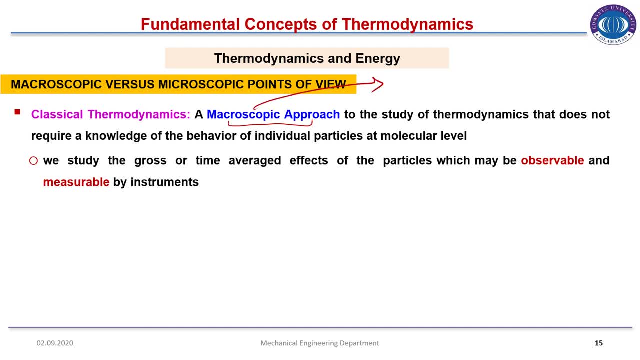 As the word suggests, macro. Macro means large, So we will deal with the large body And we will not consider our approach to the at the molecular level of the system. We will study the gross or time average effect of the particles that may be observable and measurable by instrument. 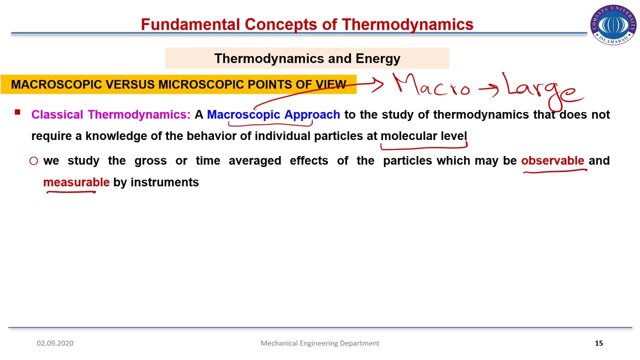 Okay, As you can see that We cannot observe the system at molecular level, So in the observable approach We will study the macroscopic approach And measurable by instruments Like pressure, volume, temperature. These are the basic properties Which we will be studying in our thermodynamics course. 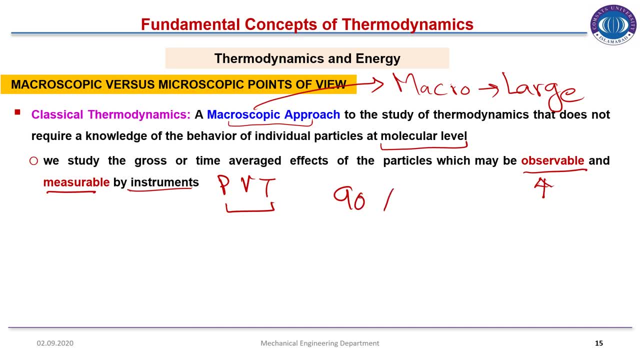 So 90% of the course Deals with the classical thermodynamics and macroscopic approach. So only 10% of our courses Deals with the microscopic approach And only 10% of our courses. So we deal with volumes that are considerably large compared to molecular dimension. 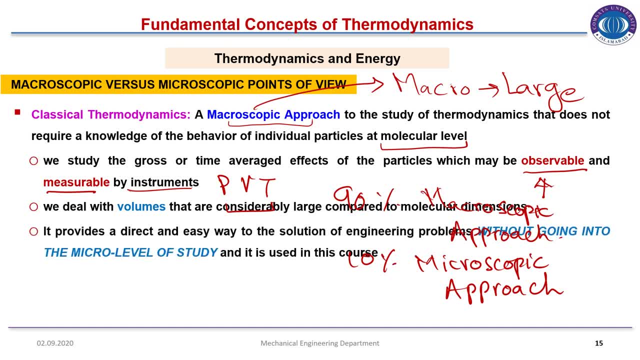 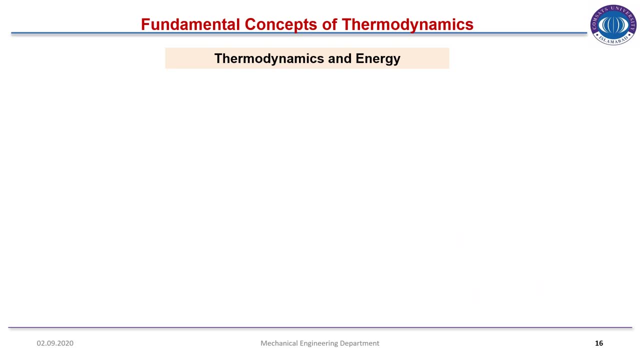 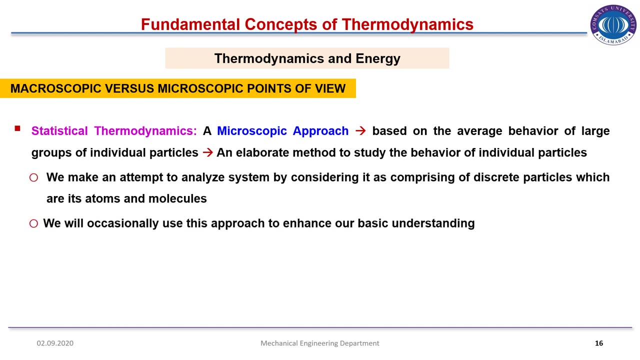 It provides a direct and easy way to solution of engineering problems without going into micro level of study, As it is used in this course. Okay Now, what is statistical thermodynamics? It is based on microscopic approach Based on average behavior of large group of individual particle. 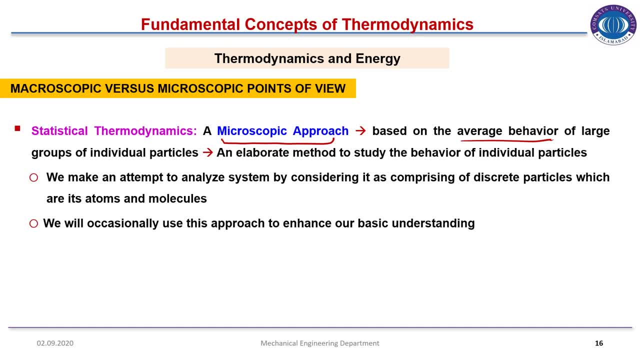 Elaborate the method of study of behavior of individual particles That are, At times, Molecule. We make an attempt to analyze system By considering it as comprising of discrete particle, Which are its atom and molecules. We will occasionally use this approach to enhance our basic understanding. 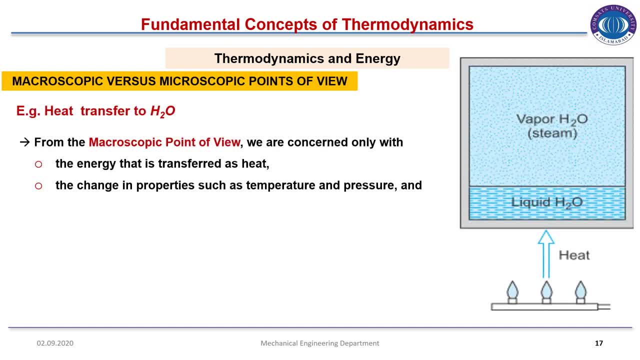 Okay, This is the Example of heat transfer to water. From the macroscopic point of view, We are concerned only with the energy that is transferred as heat, That will be Q Change in the properties, such as temperature, pressure and Volume. 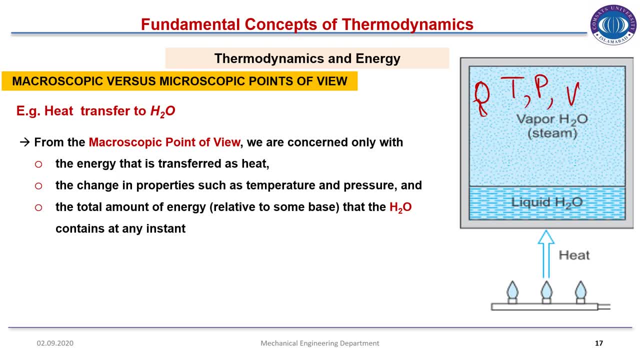 Temperature, Pressure, Volume, Amount of energy, U, Enthalpy That the water contains at any instant. Questions about how energy is stored in the water does not concerned us From a microscopic point of view. We are concerned about the way in which 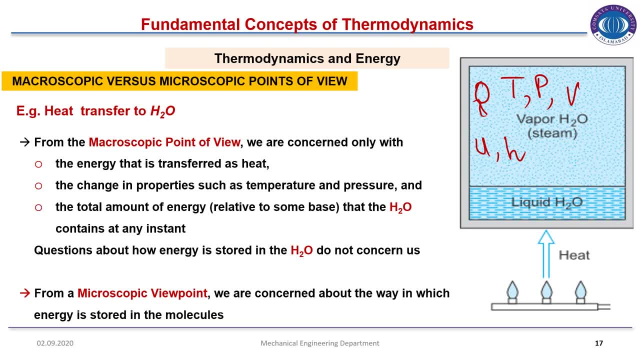 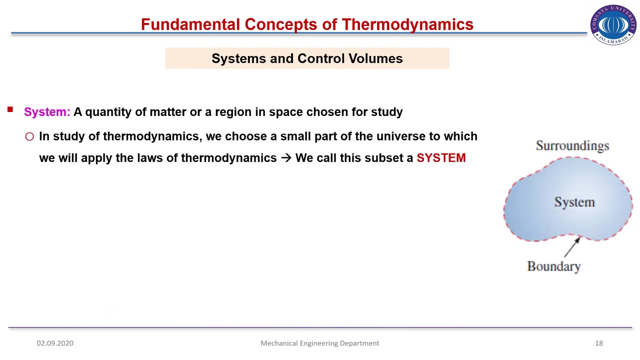 Energy is stored In the molecules Is how, How energy is stored at atomic level. Okay, This, These are some basic Definition Regarding system Surrounding and boundary. What is the system, Quantity of matter or space chosen for? 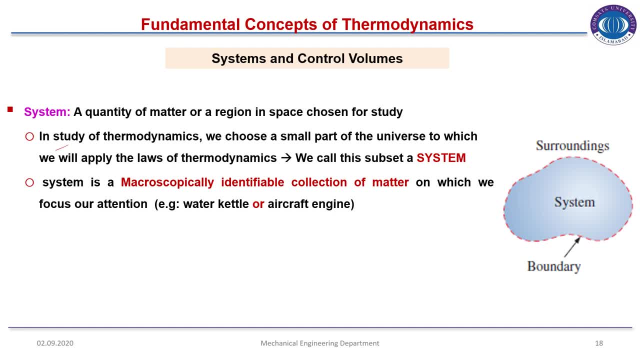 Study The space Under the concentration Or study Is. This is Is our system. Instead of thermodynamics, We choose A small part of Universe To Exist In The System, So This Part of 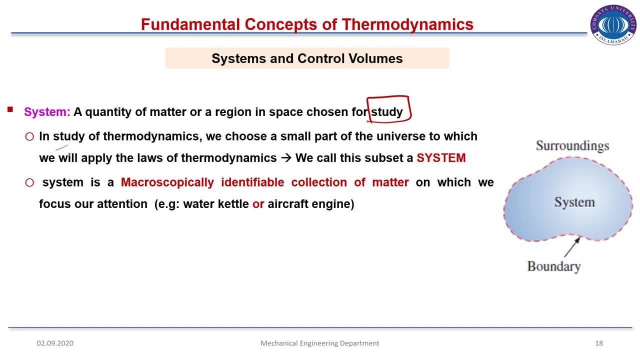 Universe To Which We apply The laws Of thermodynamics. We call This Subset A system. For example, This is a very Huge Room And We choose This Part As Our 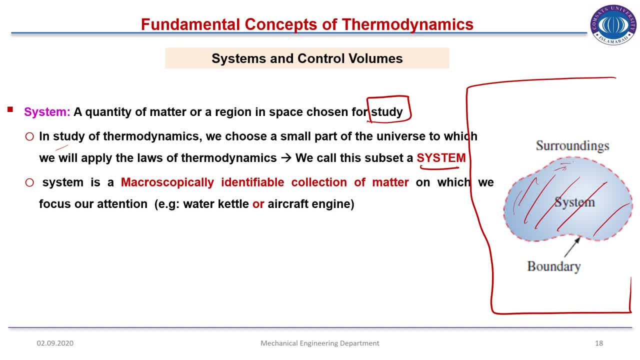 Study. So This Will Become Our System, So This Is Our System. So This Will Become Our Surrounding, The Mass Or Region Outside The System. 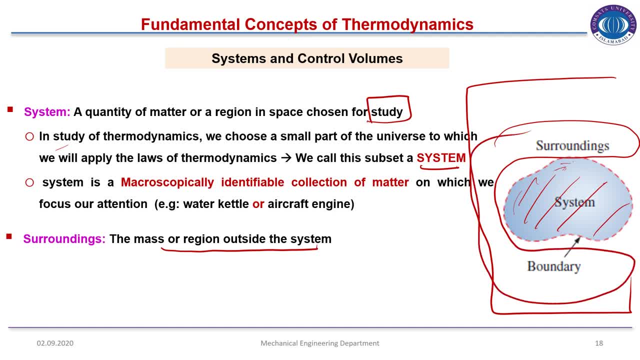 Is Called Surrounding, So This Will Become Our Surrounding. The Rest Inside The System Close Enough To The System, Have Some Participle Effect On. 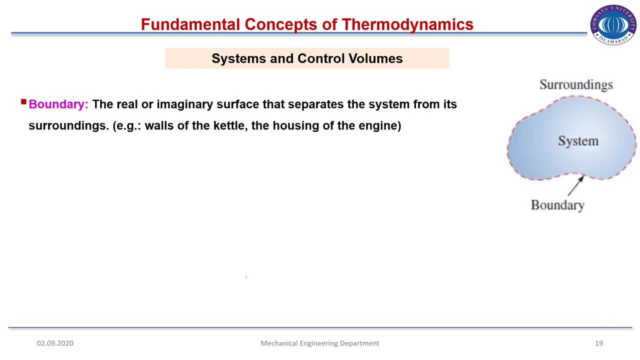 The System Is Called Surrounding A Boundary- A Boundary Can Be Real. Or Engineering Surface That The Housing For Engine A Boundary Can Be Real. 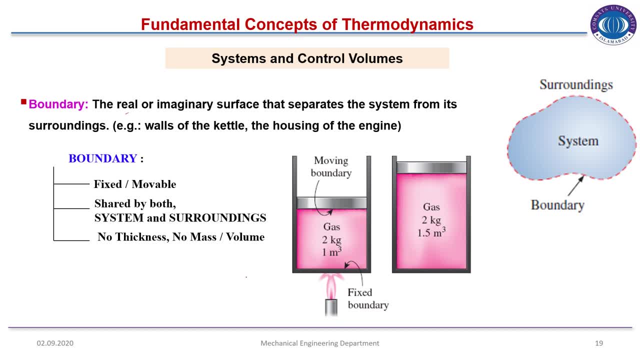 Or Imaginary. Okay, There Are Some Properties Of Boundary. A Boundary Can Be Fixed Or Movable, Shared By Both System. You Can See Here It's. 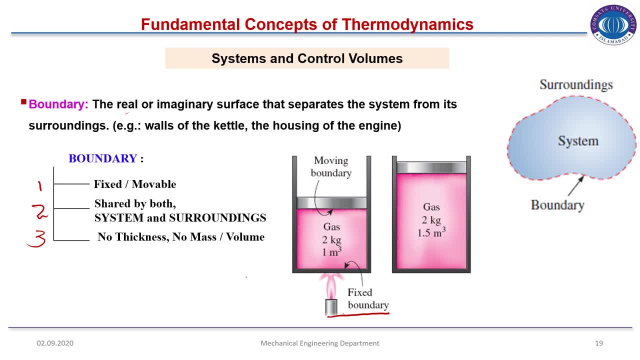 A Fixed Boundary. It's A Picture Of Piston Cylinder System. Here Is Any Gas Mass Two Kg And Volume Is One Meter. Cube Heat Is 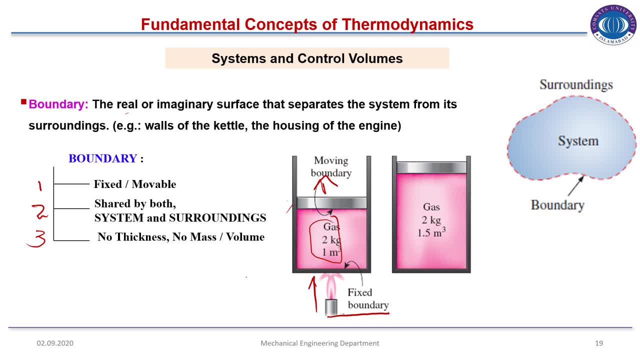 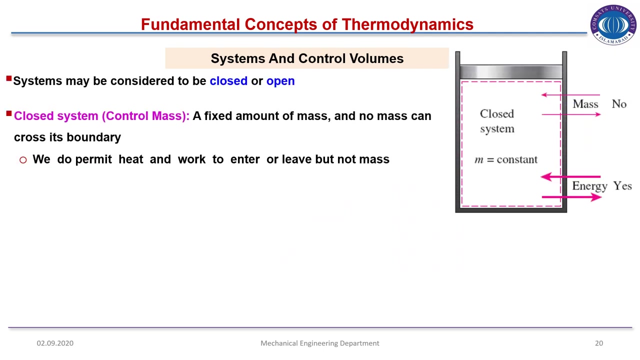 So This Are Fixed. It's Of Boundary, That Is The Movable Part Of The Boundary. Okay, There Are Two Types Of System. Okay, So There. 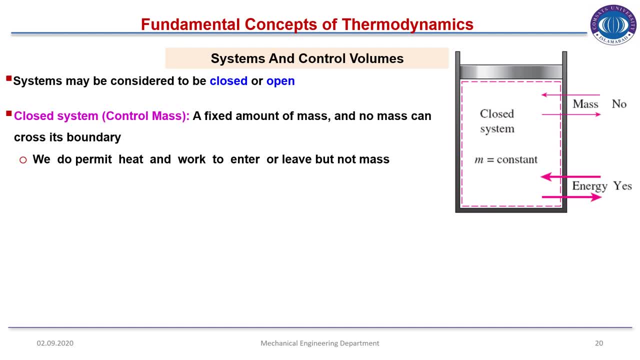 Are Two Types Of System, Mainly Close, Or One System. Close System: A Fixed Amount Of Mass And No Mass Can Be Cross Its Boundary. 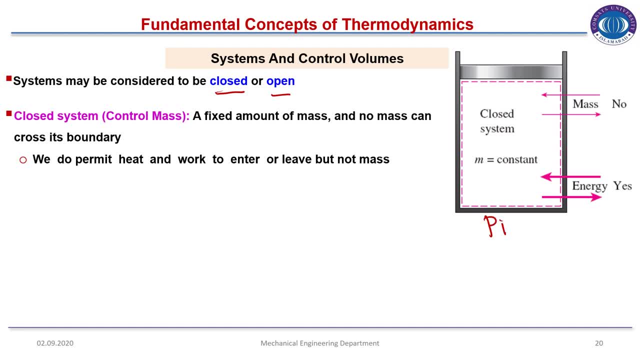 The Example Of Piston Cylinder Is Of. Piston Cylinder Is Example Of Close System Here. That Is A Movable Boundary. These Are Fixed Boundaries. 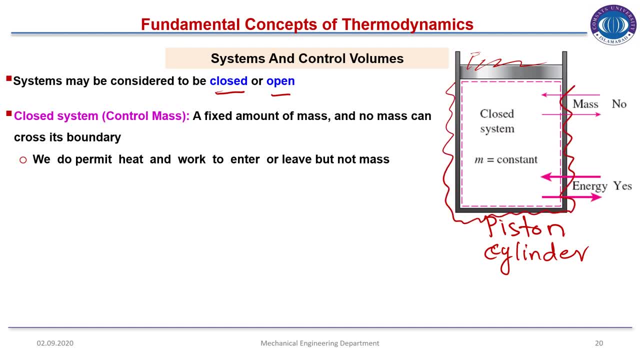 But You Can See That No Mass Can Enter Or Exit The System. However, You Enter And Leave The System At Any Point. And What Is? 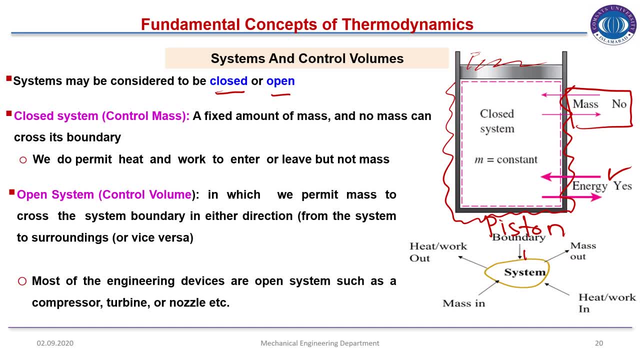 Open System. Okay, In An Open System, Energy As Well As Mass Can Is Allowed To Enter Or Exit. In Here Is A Definition Of Open. 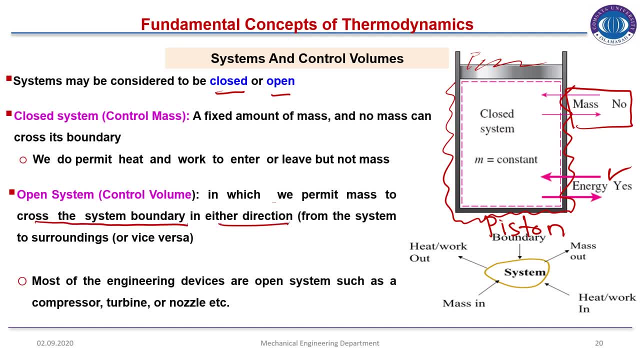 System In Which Mass Is Permitted To Cross The Boundary In Again That It Can Enter The System And It Allowed To Open System Okay. 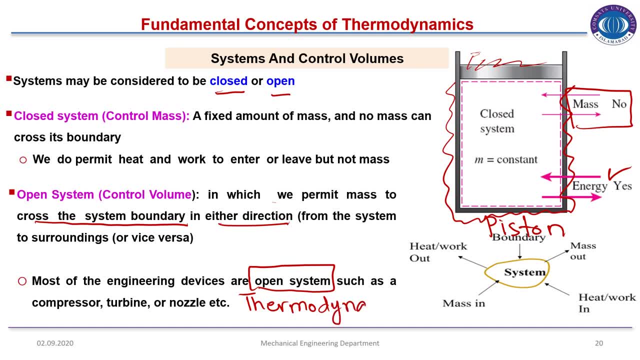 At Any Point Is Open System And Any Mass Is Allowed To Enter In An Open System. Where Is In Thermodynamics To You Will With. 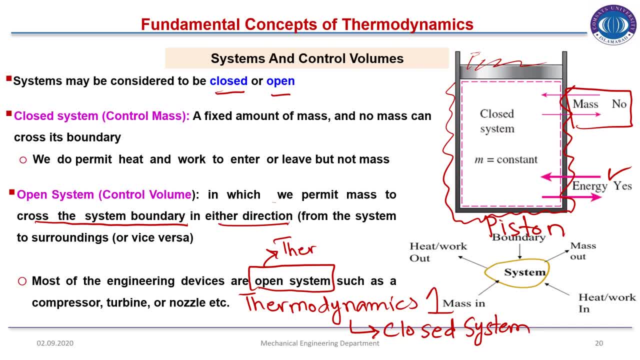 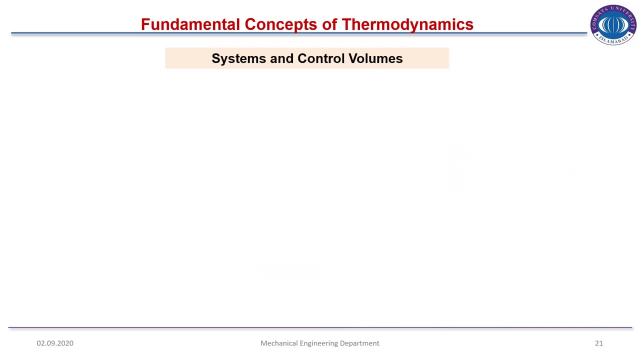 The System In Thermo Tool. You Will Study More About Open Systems And Most Of The Engineering Application Are Open System. The Boundaries Of Control. 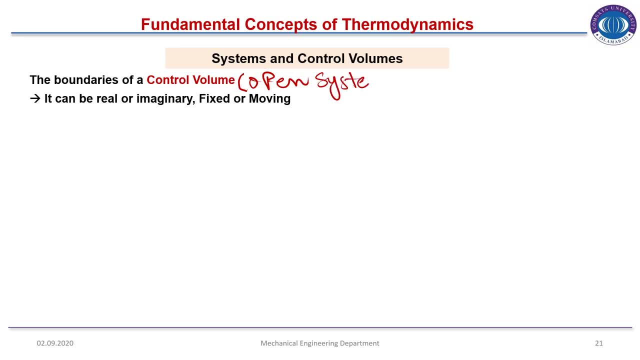 Volume, The Open System. Where This Is, There Is Mentioned Control Mass. It Means Close System. So The Boundaries Of An Open System Or Control. 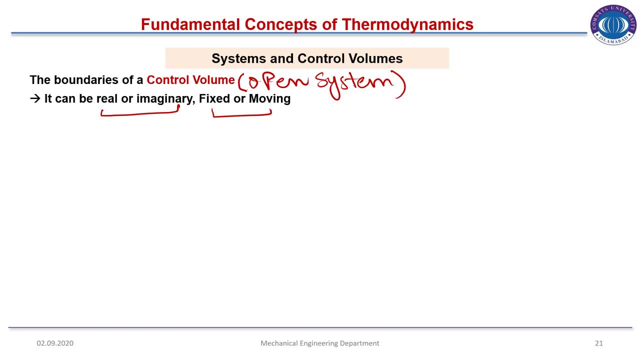 Volume System Can Also Be Real. Okay, Here You Can See A Control Volume With Real And Imaginary Boundary. This Is A Nozzle Metric Diagram. 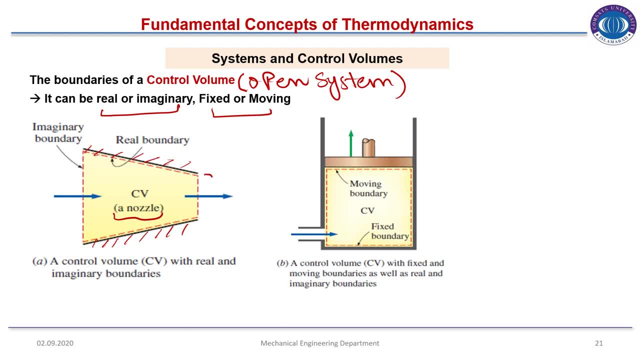 Of Nozzle. These Are Boundaries, Whereas These Are Imaginary In Open System. We Focus Our Attention At A Specific Point, So We Will Regard. 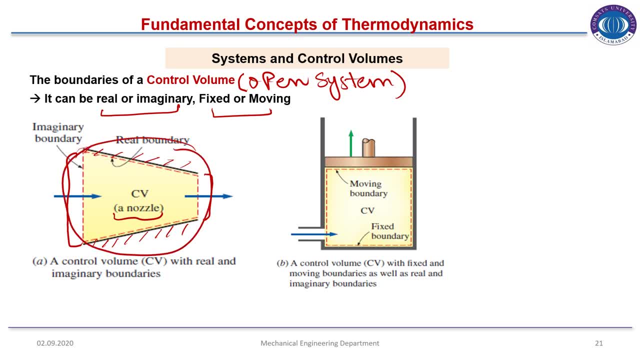 This As A System Like This Is A Nozzle And This Is A Part Of A Fixed Boundaries. Mass Is Entering From Here And 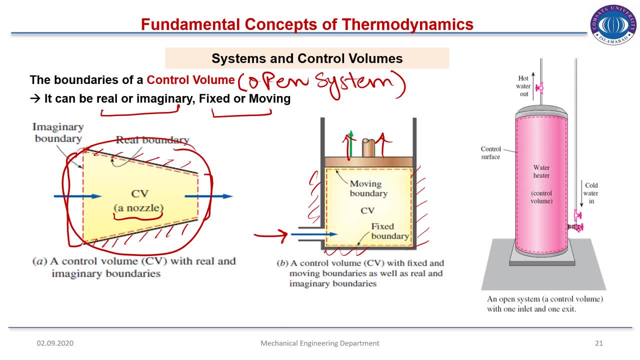 It Is Pushing The Piston Upward. This Is A Household Example Of An Open System Of A Geyser Heating Water Here And Out. 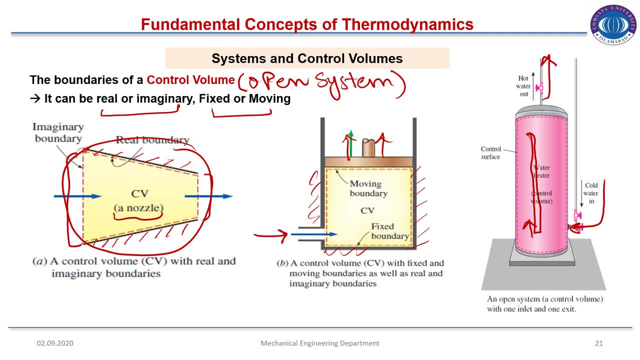 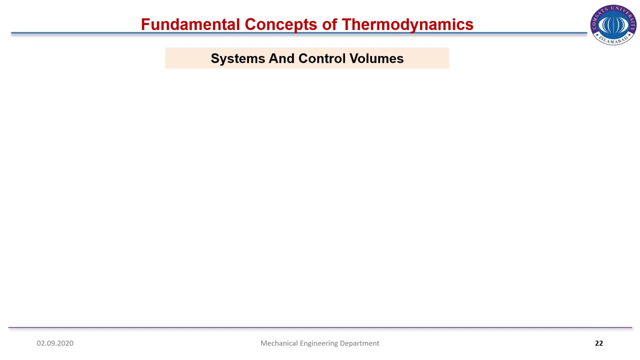 Water Leave From The Geyser Here To The Household. Okay, Well, Thank You. The third type of system is isolated system in which there is no interaction between the system and surrounding whatsoever: No mass transfer, no energy transfer. 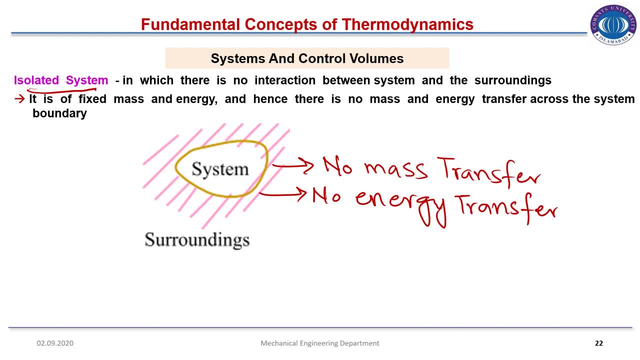 It is a fixed mass and energy and hence there is no mass and energy transfer across the system boundary. We must choose the system for each and every problem we work on so as we obtain best possible information and how it behaves. So when a problem is given to us to decide what type of term we are dealing with, either it is a closed term, open, isolated. 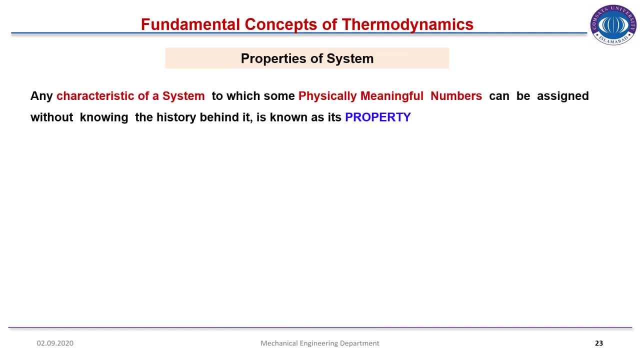 Properties of system. Any characteristics of system to which some physical meaningful number can be assigned without knowing the history behind it is known as property of the system. Example: Pressure, volume, temperature and mass, etc. Viscosity, electricity and thermal conductivity. 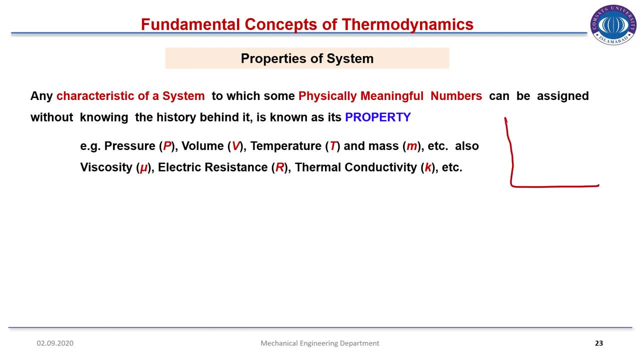 So If you have any system, That system is, let suppose is- water, At any point You can assign or you can find out with the help of any instrument: pressure, temperature威tom, viscosity, mass Balance. these are properties of the system. these properties are classified into two. 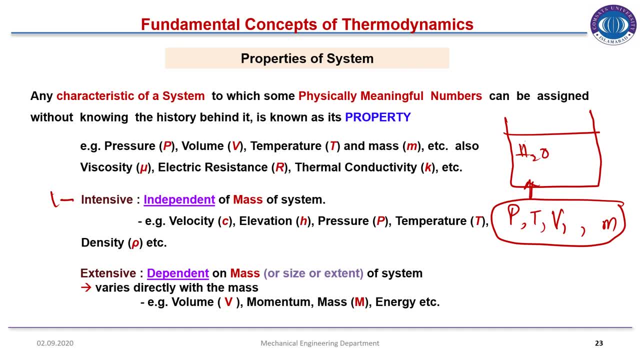 basic types with intensive property and the kids, except property. intense properties are independent of mass of the system- example: velocity, action, pressure, temperature, etc. whereas extensive properties depend on the mess or size or extent of the system. where is directly with the mass- example: volume, momentum, mass, energy etc. 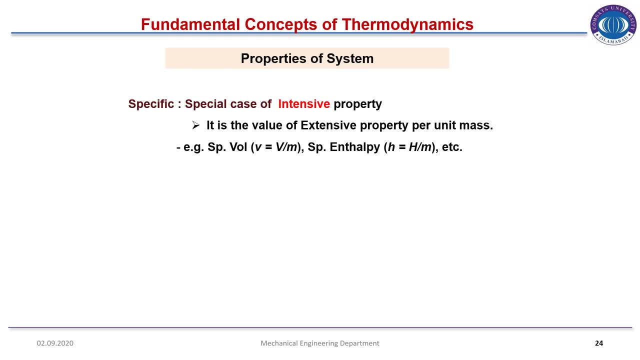 there are some specific properties as well. specific properties: these are very important in our subject. ok, this is a special case of intensive property. it is the value of extensive property per unit mass. as in the previous slide, we have studied that extensive properties depend on the mass, like volume. 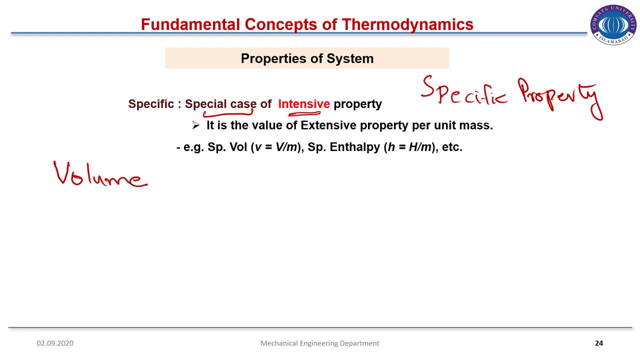 uum tense property. So it is written that a tense key is a specific property, Extensive property. divided by this is a specific property Like specific volume, specific enthalpy, specific internal. All these are the specific properties of the system. Extensive properties per unit mass, such as 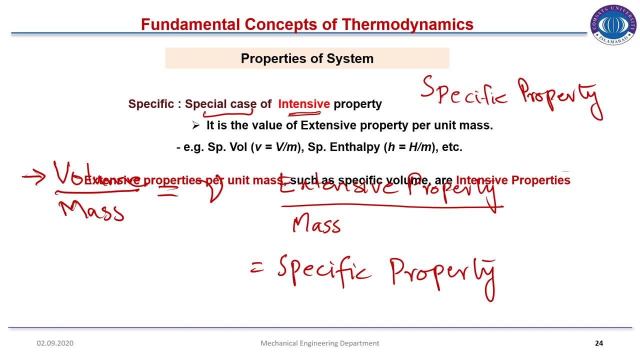 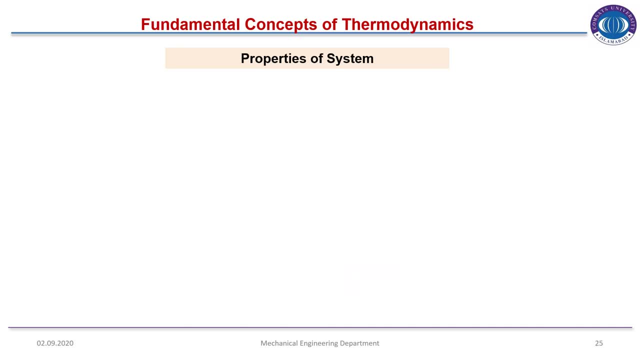 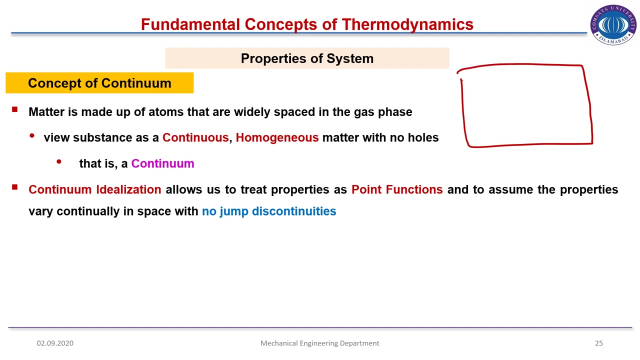 specific volume are intensive property. Now we will discuss about the concept of continuum. Matter is made up of atoms that are widely spaced in the gaseous phase. We view the substance as a continuous, homogeneous matter with no holes. That is the concept of continuum. Now, 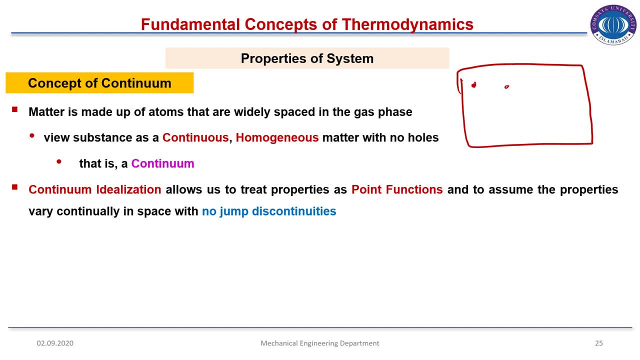 we know that in gaseous phase the distance between the molecules is very large, But the concept of continuum states that these molecules are in continuous and homogeneous matter with no holes, no space between atoms. Continuum idealization allow us to treat property as point function. 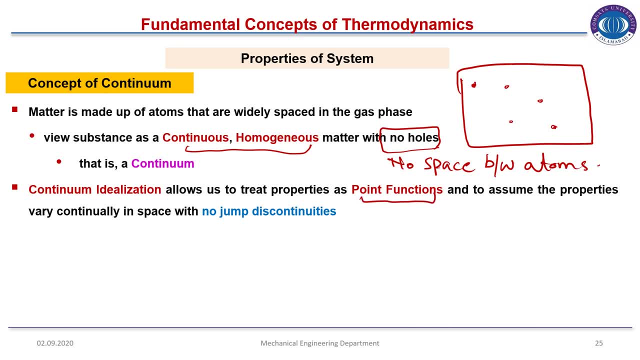 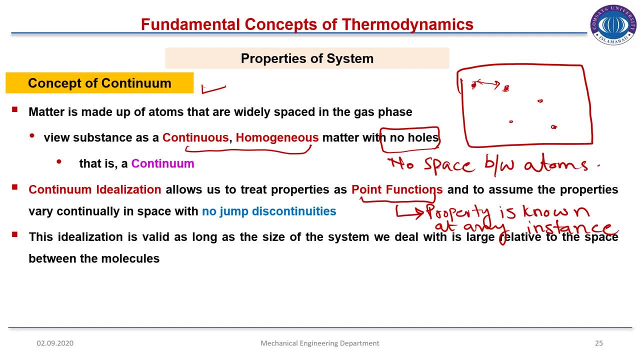 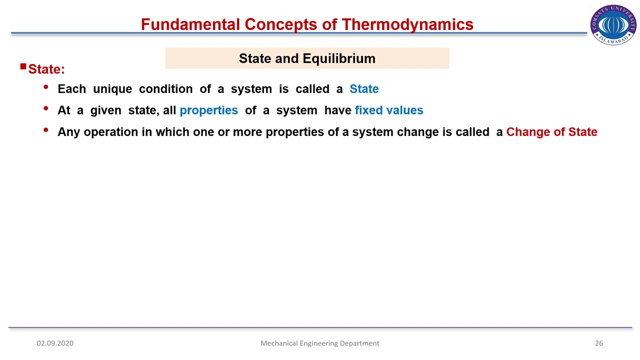 is large relative to the space between the molecules. this is the case in practically all problems. we will limit our consideration to substance that can be modeled as continuum. so in the in our course, all the systems we will study are the continuous system state and equilibrium state. each unique condition of system is called state at a 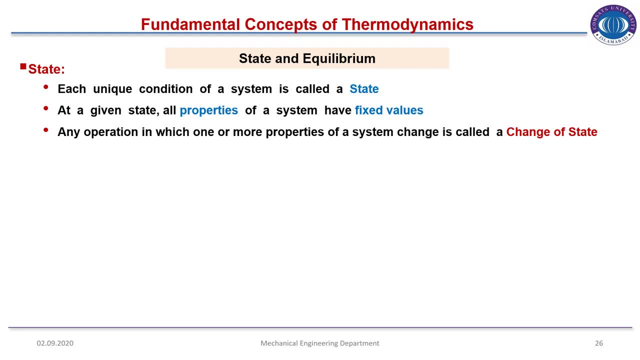 given state. all properties of system have fixed values. any operation in which one or more properties of system change is called change of state. for example, we have state 1 and state 2. a state 1, we have pressure P 1, T1.. At state 2, we have pressure P2 and temperature T2.. So at state 1, the value of P1 is fixed. 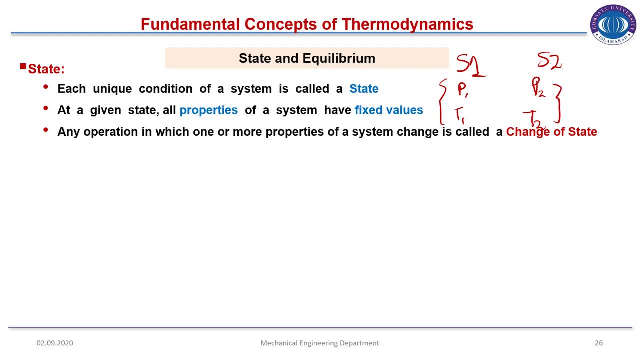 and T1 is fixed At state 2, the value of P2 and T2 is fixed During the change from pressure: P1 to P2, this is known as change of state- and T1 to T2.. Temperature will be changed from state 1 to state 2.. So thermodynamics deal with the equilibrium state. So what? 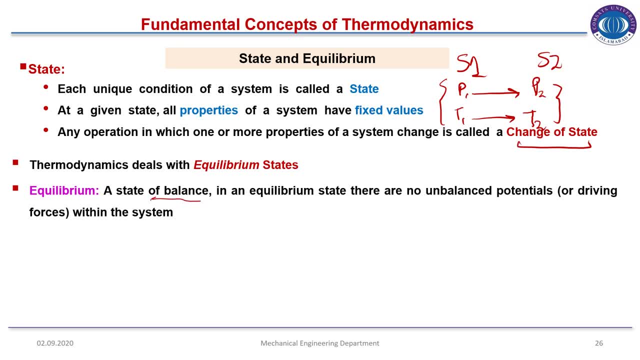 is equilibrium, A state of balance. In equilibrium state, there are no unbalanced potentials or driving force within the system. There are three types of equilibrium: Thermal equilibrium: if temperature is same throughout the system, Del T is equal to zero. In mechanical equilibrium, there is no change in pressure at any point. 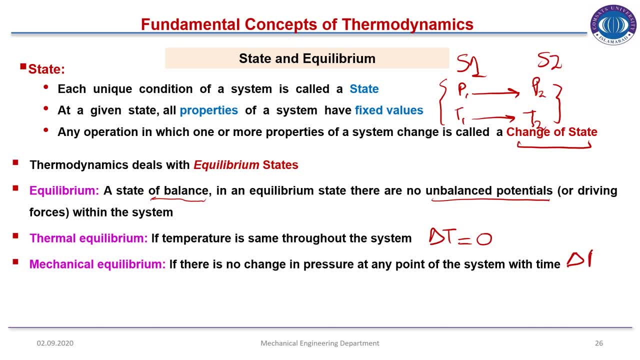 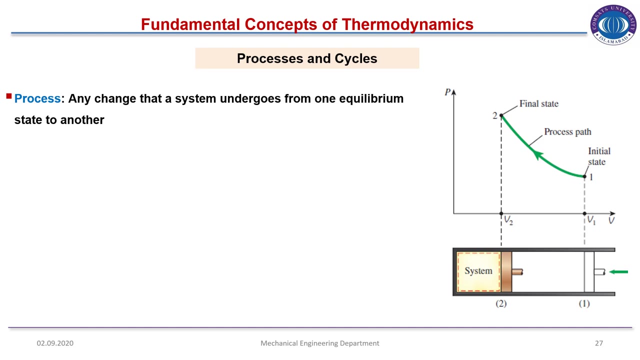 of the system And in phase equilibrium. if a system involves two phases and when the mass of each phase reaches an equilibrium level, it stays there. So phase is an equilibrium, cycle Processes and cycle Process: Any change that a system undergoes from one equilibrium state to another is known as process. 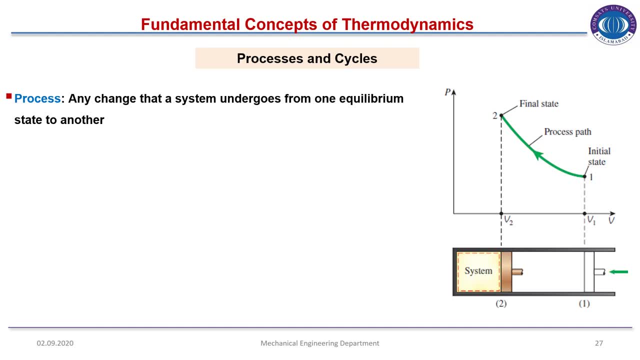 So here is the pictorial view of process. It's a P-V diagram from state 1 to state 2.. There's a processes happening And the there is. that is the change in the cycle and with that change, This is the process: prolongation, G and V cost. It depends on the system and system. Finnish: vorher frei bridgenamdada那個 وبождиеy int까지csamadaagetur. 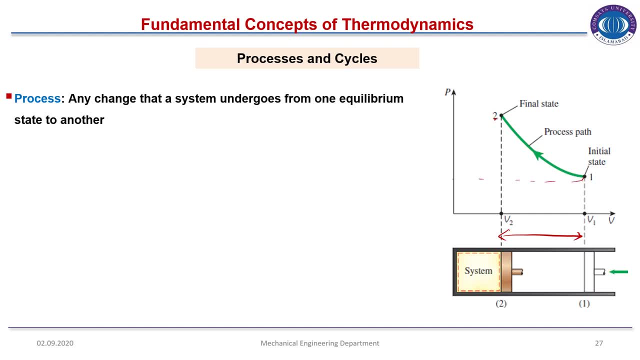 volume, and that is the change in pressure, is a piston cylinder, the volume is reducing. the initial volume was that and it is reduced by this. this is the final volume. path, series of states through which a system passes during the process, is known as path of the system. to describe a process completely, one should specify: 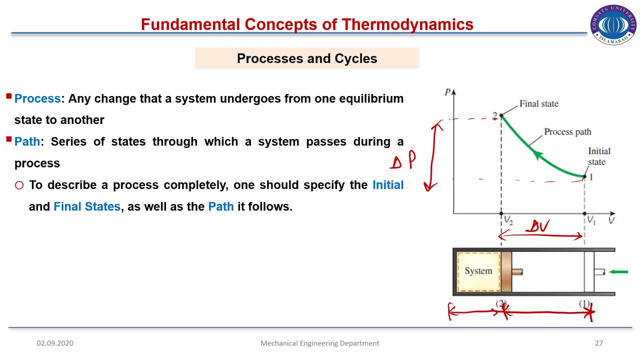 the initial and final states, as well as path it follows, to know the create information. we should know about the initial state, that is, state 1, the final state, state 2- and the path which it follows. we should know about all of these things to know the process. 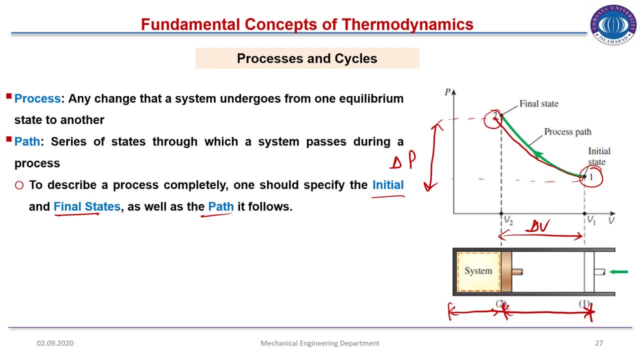 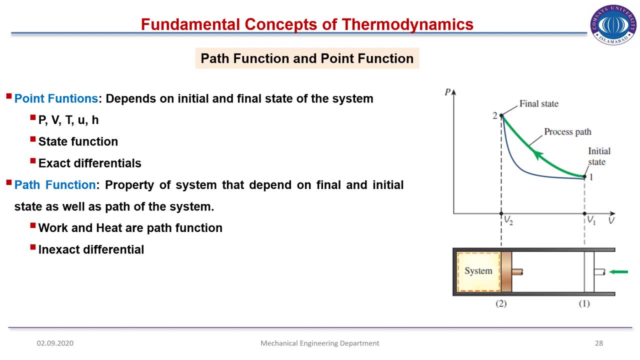 completely path functions and point functions. what are point functions? point functions depend on final states only. these include pressure volume and the final state, temperature, tenor, energy, enthalpy. these all are state function and exact differential. what is meant by exact differential is that, if you know, we 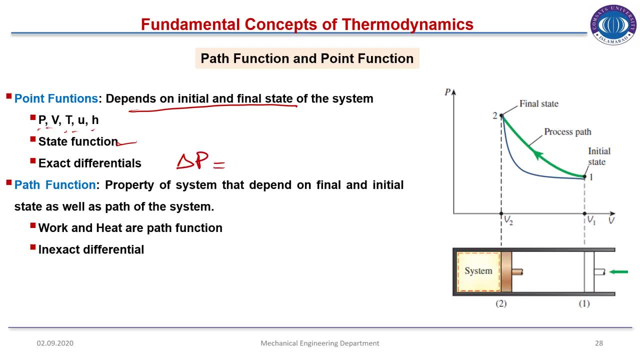 want to know the value p. you know it's about your pressure at point state 2 and you know the exact value of accommodate point three. point a, point state 1inesice & Eывать of y- thankful isakoo记记 news. audience areไม่опмотри. and answer. you do not see now if its known. so that if you want to know the value of p, please read the articulation at 2 and your share is printed on your screen. state 1: the vehicle is selected and mixed tone must be posted so that the value of 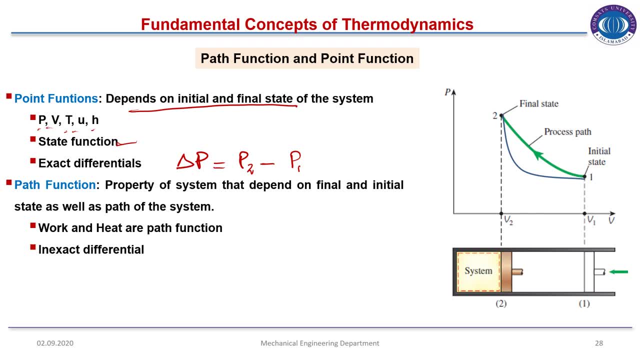 extreme好ит فارmount being maintained will be registered by Byron in order tomen- you know it, bottom quite well- to obtain control over of knowledge is that certain size, state 1, you And what are path function? Property of system that depends on final initial state, as well as path of system. Work and heat are path function. 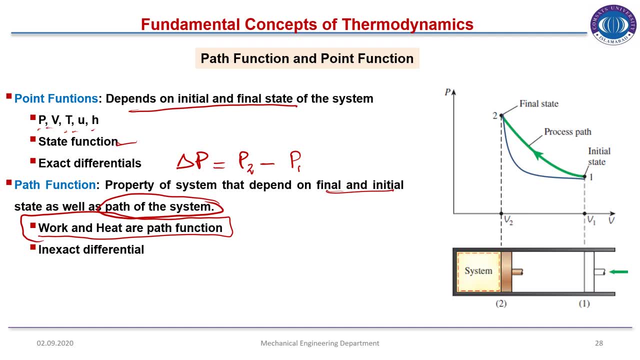 Usually this, sometimes this statement in the MCQs as well. work and heat are both are path function that are not point function. They depend on the path followed by the function Process during from going state 1 to state 2 and these are in exact differential. 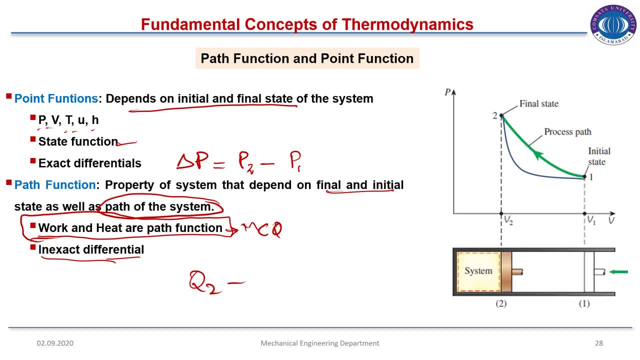 You cannot find the value of Q minus Q. Same example is shown here: Cylinder system. The cylinder contains pressure fluid and the piston move from state 1. To state 2. The volume is reduced And the pressure is increased. But now you can see that this path 1 and this is second path, the initial and final state are same. 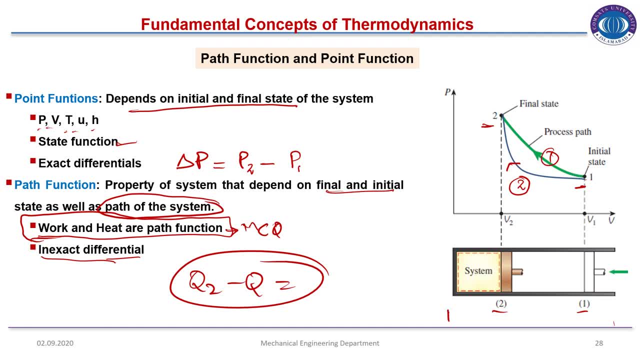 But the path followed is different. So the amount of work and heat in the process path 1 will be different from process path 2.. So at the end we have the final state. So we have initial and final state And, as you see, we have the final state. 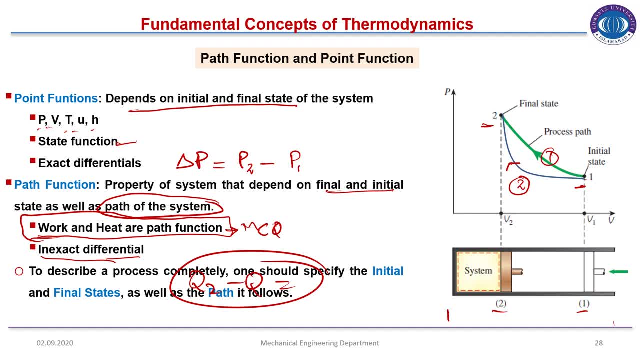 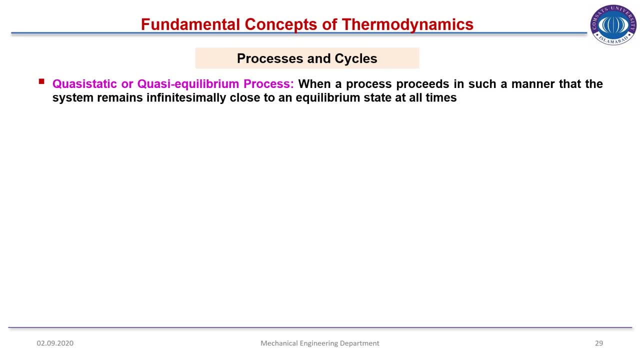 So to describe a process completely, one should specify the initial and final state, as well as path it follows. Causized static and Causize equilibrium process. Causized static and Causize equilibrium process. When a process proceeds in such a manner that the system remains infinite, the smell of the process will disappear. 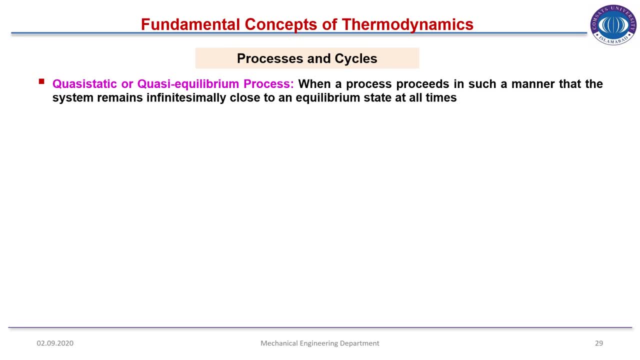 infinitesimally close to the equilibrium state at all time. the process is known as quasi static or quasi equilibrium process. okay, so when the word quasi static or quasi equilibrium come. you should know, that is a very slow process. piston is moved slowly, molecules will have sufficient time to redistribute and 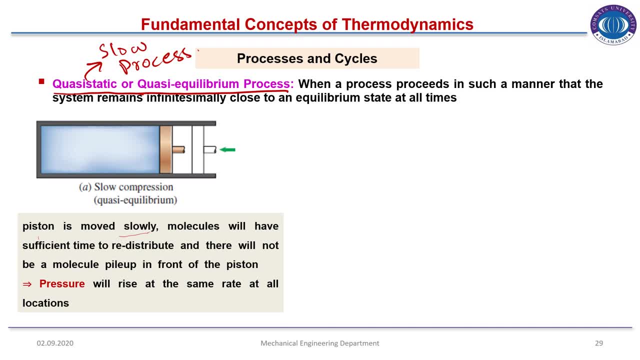 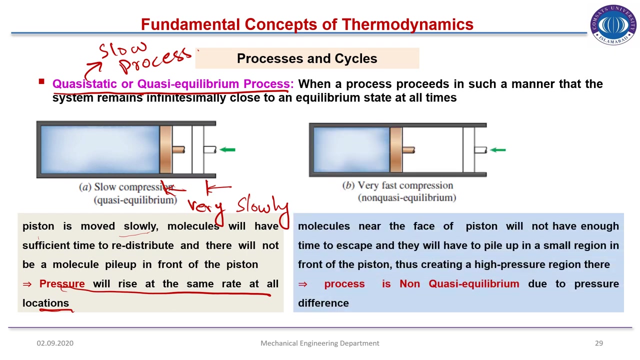 there will be. no, there will not be a molecule pile up in front of the piston. pressure will rise at the same rate at all location. piston move from this point to this very slowly. so this is the quasi static or quasi equilibrium process, and its opposite is non-quasi equilibrium process. that is fast process. and what is the disadvantages of? 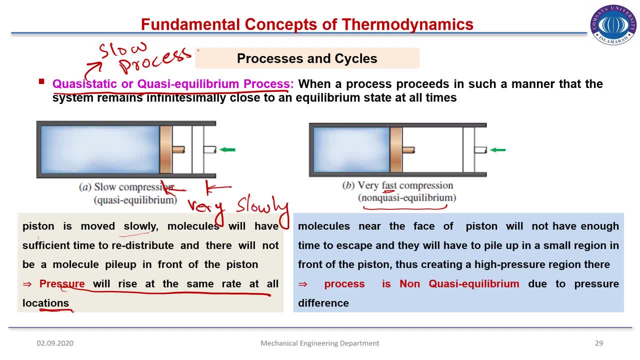 non-quasi equilibrium process molecule near the face of the piston will not have enough time to escape and they will不錯 pile up all region, creating a high pressure region. so there will be no equilibrium. in a fast compression process is known as quasi equilibrium due to pressure difference. non 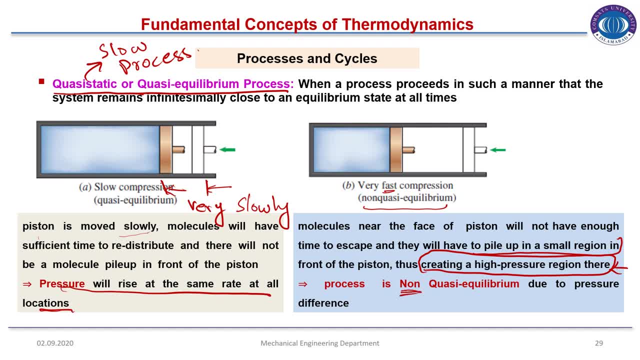 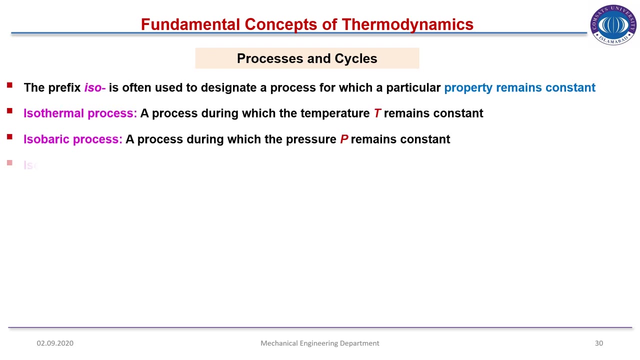 cause why? so? this is cause I slow and for fast, that is okay. processes and cycle, and you know the prefix ISO, so used as to design process that for which particular property remain constant. example: isotherm process in temperature remain isoic. process in which pressure in correct process, in which volume in constant, so early isentropic process, isentropic. 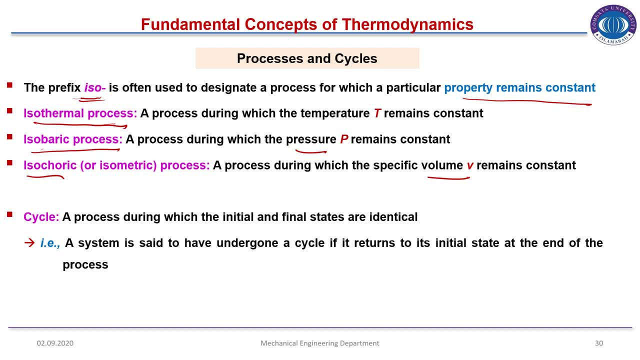 process in which entropy remain constant and in which enthalpy remain constant. Cycle processes during initial and final stages are identical. We will see in the next slide. A system is said to have undergone a cycle if it returns to its initial state at the end of the process. 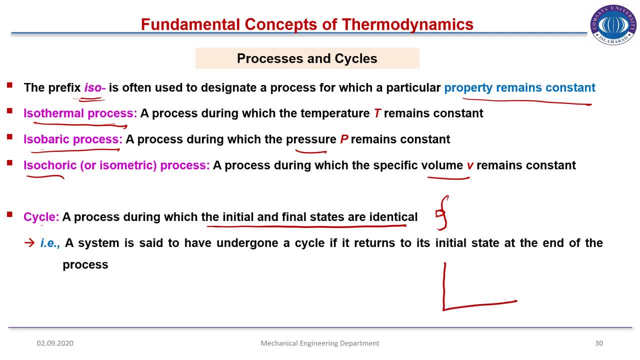 For example, the process, that is, one that state 2 system goes first from state 1 and then goes back to state 2, 1, from 1 to 2 and then back to state 1.. This is known as cycle, cyclic process. 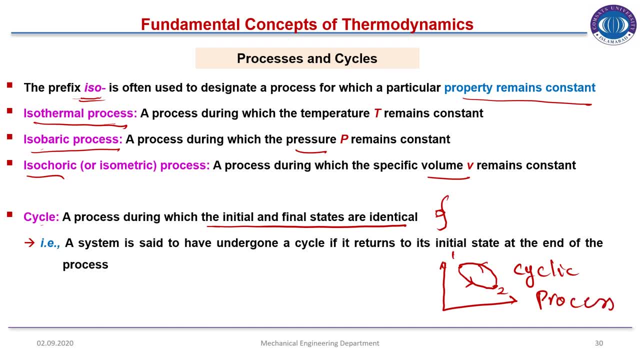 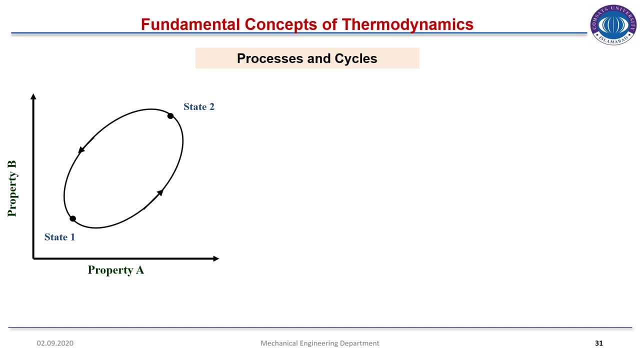 So this is the cycle. Some processes are shown. This is the figure 1.. Cyclic process is shown How it is cyclic. The process starts from state 1 and from this path it moves to state 2 and it comes back. 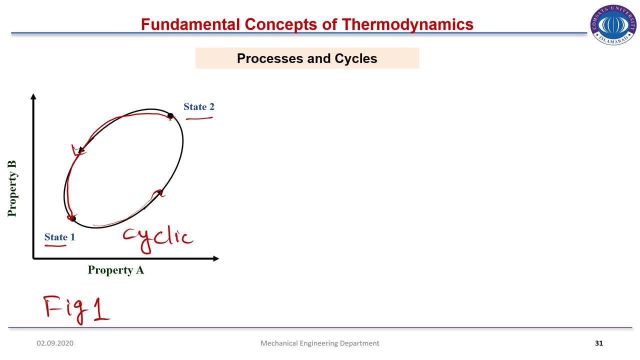 to its initial state, state 1 in a cyclic process. This is the volume versus pressure P-V diagram. This is two. In this isochoric process and isobaric process are shown. Isochoric process is a constant volume process. 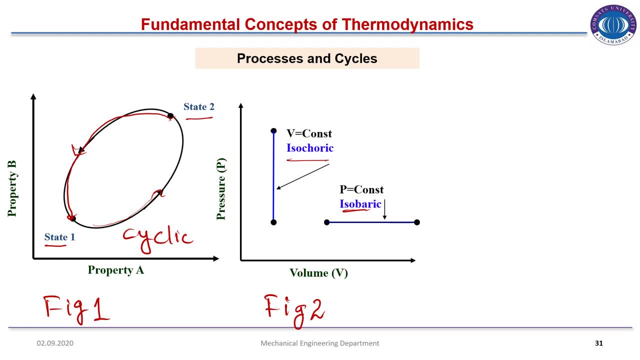 So it is straight line in parallel to Y axis. Isobaric process is a constant pressure, So it is a straight line in parallel and in y axis processes. and if this is also a straight line, parallel to x-axis temperature versus entropy, so isothermal process is a constant. 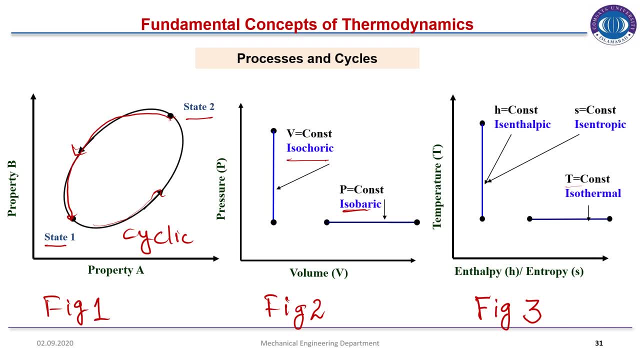 temperature constant process. this is a straight line parallel to x-axis, you can see, and isentropic or isentropic process: in isentropic process it's a constant entropy process, as isentropic process is a constant enthalpy process. so it is a straight line parallel to y-axis: entropy and 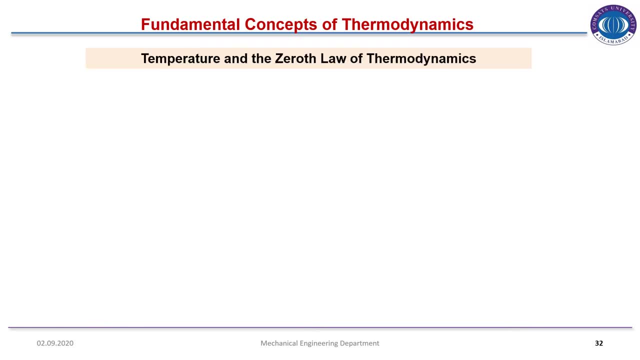 enthalpy remain constant throughout the process. temperature and the zeroth law of thermodynamicsstatement of zeroth law of thermodynamics: if two bodies are in thermal equilibrium with the third body, they are also in thermal equilibrium with each other. so here you can see. 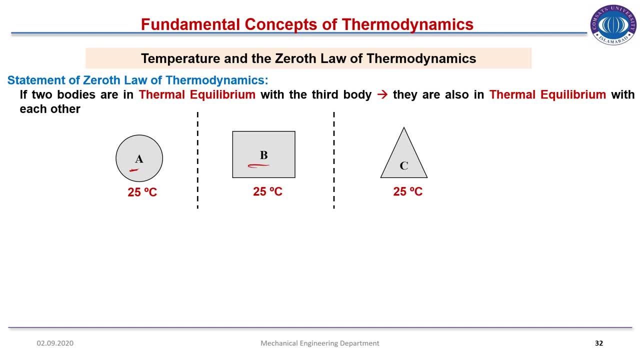 there are three bodies: a, B and C. if you see that body a is in thermal equilibrium with body B and body B is thermal, is in thermal equilibrium with body C, then always should be on thermal equilibrium. if body B and body B should, body a is also in thermal equilibrium with body c. this is the zeroth law of thermodynamics. 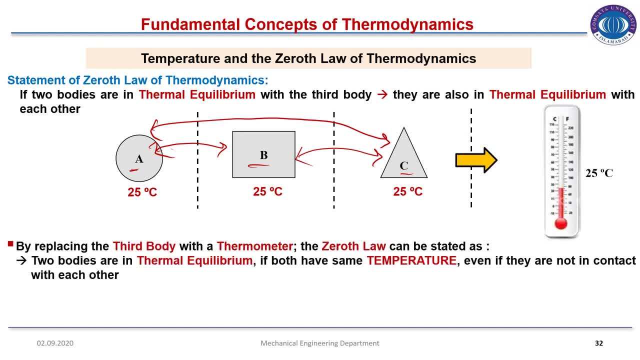 by replacing the third body with a thermometer. the zeroth law can be stated as two bodies are in thermal equilibrium if both have same temperature, even if they are not in contact with each other. so we have replaced the third body with the thermometer and the temperature and the thermometer you can see is also 25 degree centigrade. temperature of first body is 25 and 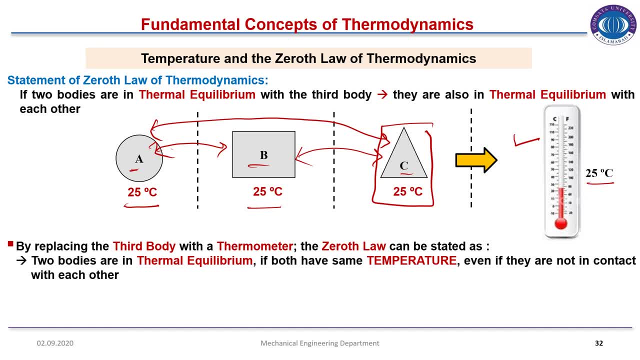 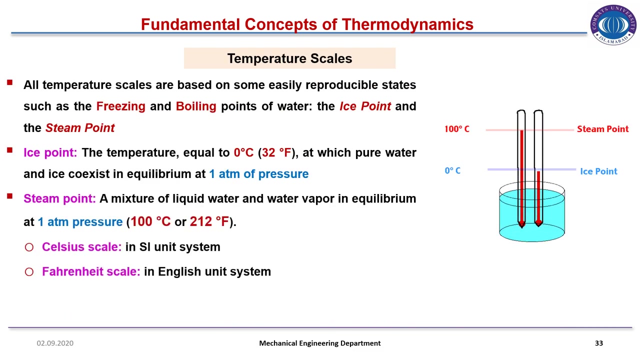 body b is also 25, so all these are in thermal equilibrium with each other. temperature bear an important relation to thermodynamics, as force does to static orientations, velocity does to dynamics. So temperature difference is the driving force in thermodynamics. Temperature scales: All temperature scales are based on some easily reproducible states. 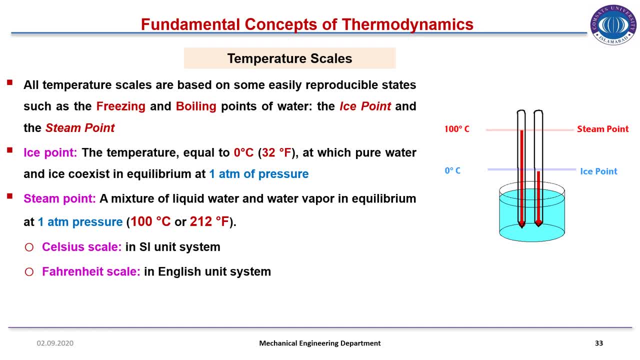 such as freezing boiling points of water, the ice point and the steam point, As you know that the ice point is 100 degree centigrade and the steam point is 100 degree centigrade. Ice point temperature equal to 0 degree centigrade or 32 F, at which pure water and ice co-exist. 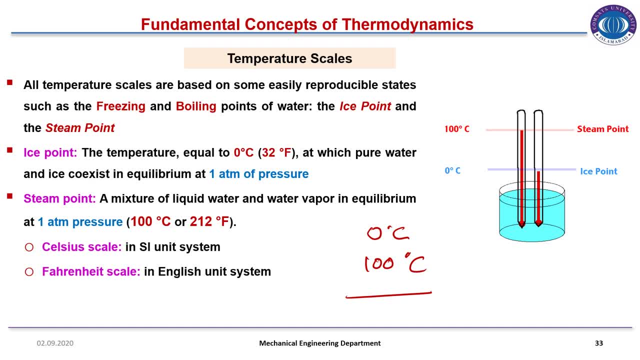 in equilibrium at one atmospheric pressure. Steam point, a mixture of liquid water and water vapor in equilibrium at one atmospheric pressure, that is, at 100 degree centigrade or 212 F. There are two main scales which we follow: Celsius scale and Fahrenheit scale. 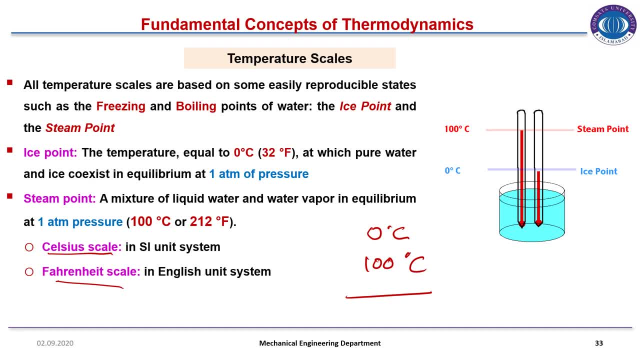 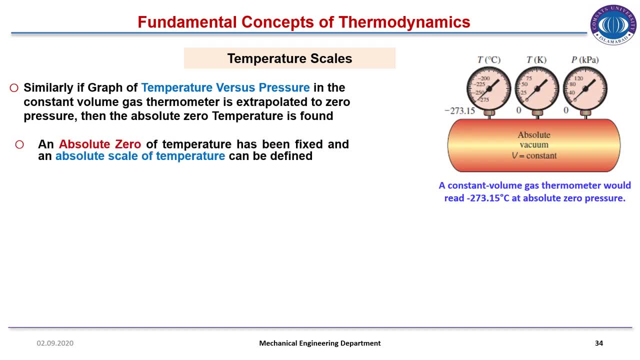 During our study, If it The main, focusing on our attention to Celsius scale. If we plot a graph of temperature versus pressure for constant volume gas thermometer, this is a constant volume gas thermometer shown here. So how this device work is that when you 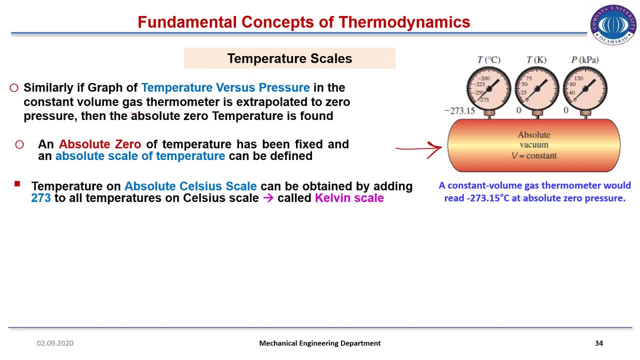 Increase the pressure, the temperature also increases. and when you reduce the pressure, the temperature also reduces. So by measuring the pressure you can calculate the temperature as well. Gas thermometer extrapolated to zero pressure, then the absolute zero temperature is found. 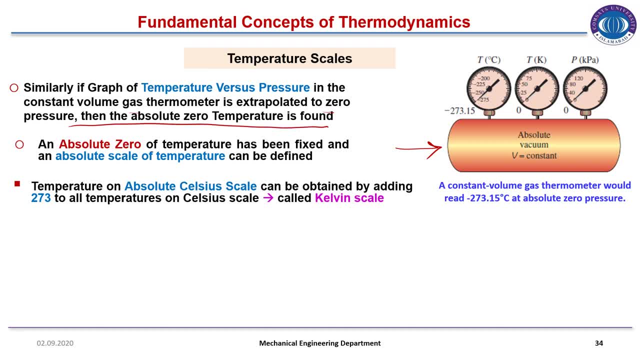 How absolute zero temperature is found, that we reduce the pressure to zero and absolute zero of temperature has been fixed. An absolute scale of temperature temperature can be defined. temperature on absolute Celsius scale can be obtained by adding 273 to all temperature on Celsius gain, that is. 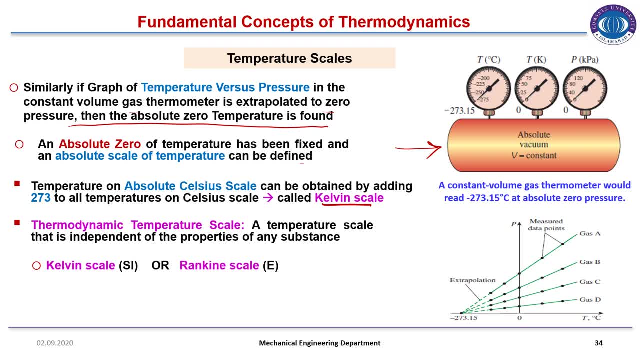 known as Kelvin scale. so, for example, if the temperature is 10 degrees centigrade and you have to find this in Kelvin, then you have to simply add 273 plus 10 to 83 Kelvin. in almost all of the problem, we will use the Kelvin scale in our 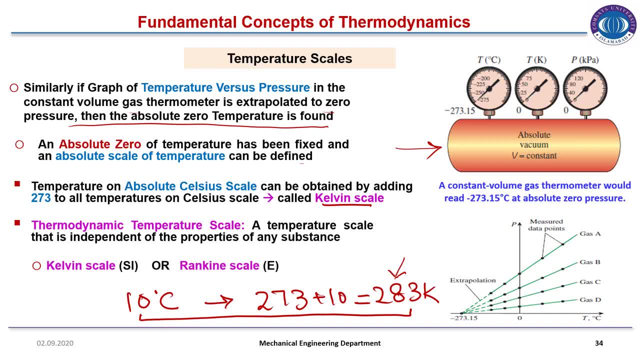 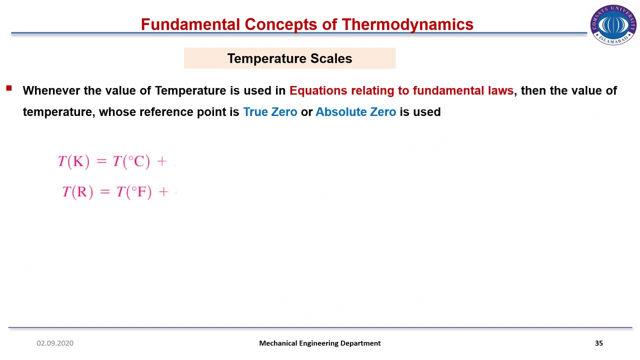 problem solving thermodynamic temperature scale, a temperature scale that is independent of property of any subs substance. this scale does not depend on the properties of substance. that is a Kelvin scale or Rankine scale. we will be using the Kelvin scale during our studies whenever the value of temperature is used in equations. 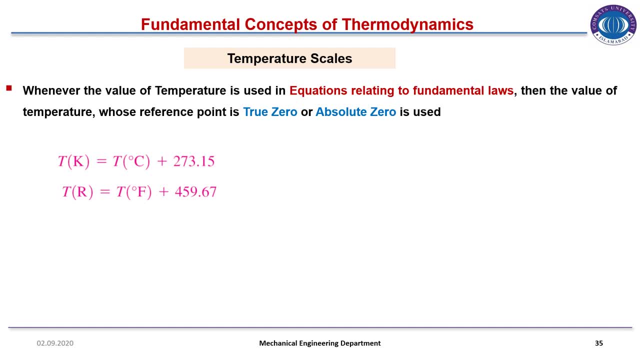 relating to fundamental laws, then the value of temperature, whose reference point is the true zero or absolute zero, is used. so we will use the Kelvin scale to find the source Flate for any certain variables where r is equal to fa and x is equal to P. but then we simply add 274 to the volume value in the-ٹ scale. so these are the relation. to find the temperature in Kelvin scale, random when scale, we will simply add 273 to the temperature which is given to us in centigrade scale SCALE. okay, the difference between Kelvin scale and Centigrade scale is: did not? accidentally change the Nanosis because of the energetically higher coolant by the process. so if I said you know the temperature very few times in a interested boy, suppose that the temperature cannot simply forget now of an example present in over time because of the recent, the current model, if we are 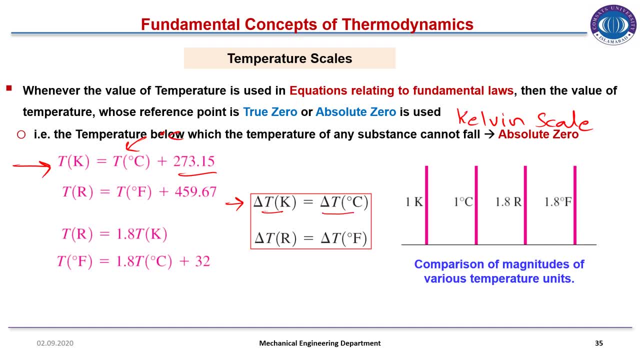 using the instrument in terms of cooling and computing power. we anybody not know how to name this. when the scale will replace between the temperature is same and the difference between Rankine scale and Fahrenheit scale is same. so these are the relation to find the temperature in Kelvin scale and. 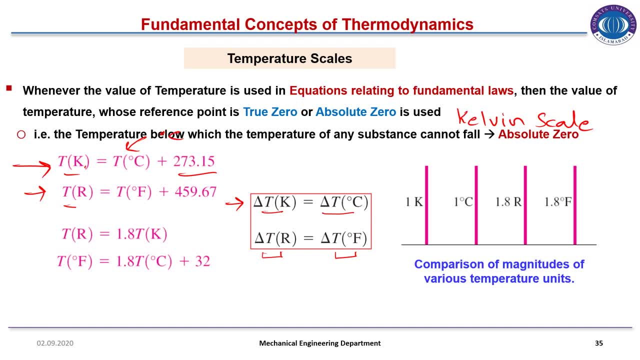 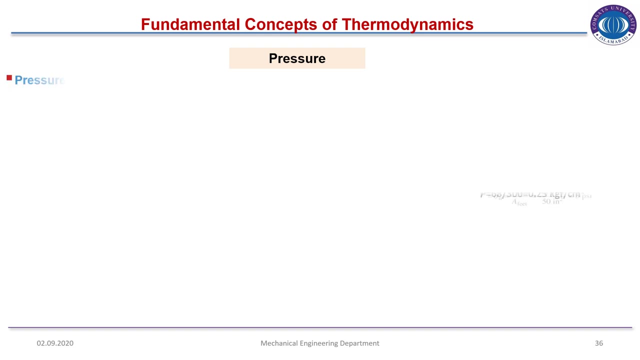 Rankine scale and between Rankine and Kelvin scale, Fahrenheit and Celsius scale. and that is the difference for magnitude of the temperature units: Kelvin, Centigrade scale, Rankine and Fahrenheit scale. okay, pressure: a normal force exerted by fluid per unit area is known as pressure. 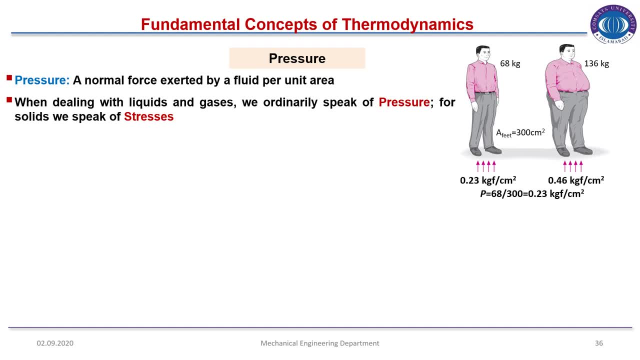 when dealing with liquid and gases we ordinarily speak of pressure. for solids we speak of stresses. in our studies, liquid pressure will be mentioned in our problem solving. so you can see there are two person standing, person 1 and person 2. the weight of person 1 is 86 kg. 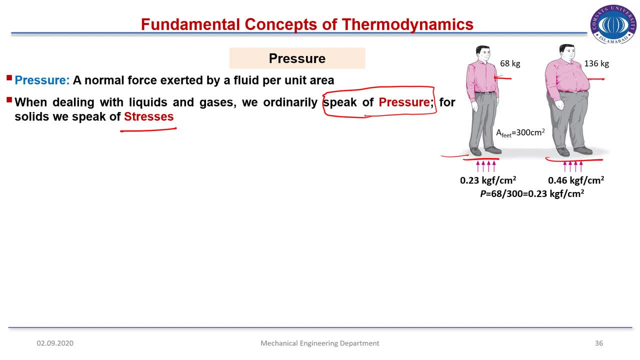 the weight of second person is 136 kg. so the resistance offered by the floor is also known as the pressure. so you can see that the pressure offered by the floor first person is 0.23, where the pressure offered by the floor the second person, who is heavier than the first person, is greater than the first pressure of the 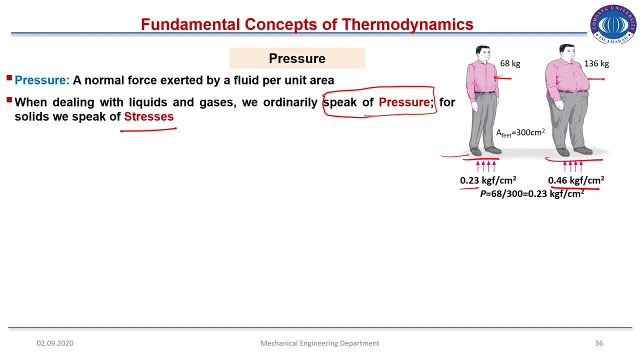 first person, that is it for six kilogram force per centimeter square. so there are some units regarding the pressure, these are SI unit and these are initials we will use in SI units for our problem solving in a problem. usually the pressure is given a Pascal, kilo, Pascal, mega, Pascal bar atmospheric. so these are. 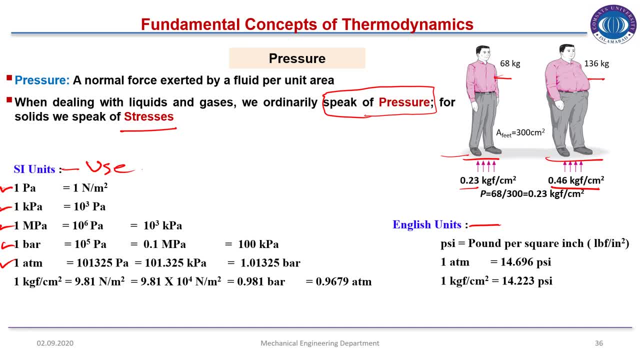 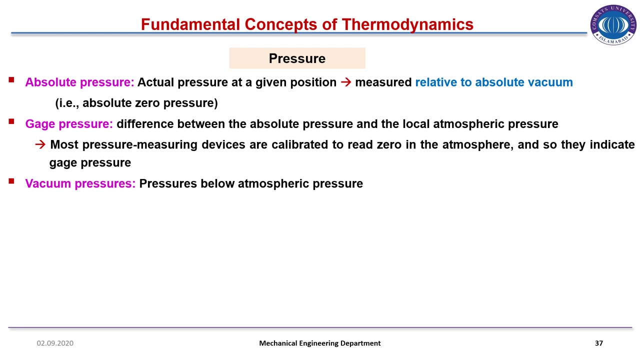 the relation how you can convert from one bar, as one bar is equal to one zero one hundred kilo Pascal. it's equal to one zero one kilo Pascal. basically so, there are three types of pressure you should know about: absolute pressure, gauge pressure and vacuum pressure. absolute pressure is the actual pressure.